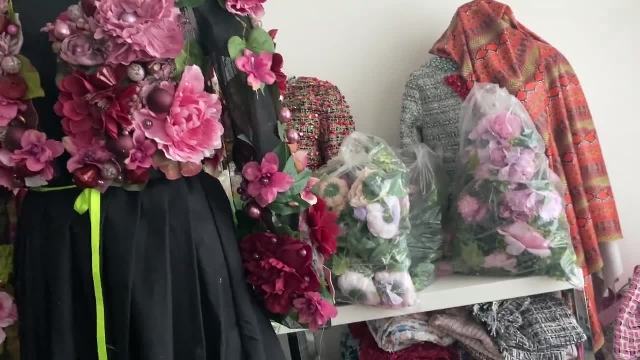 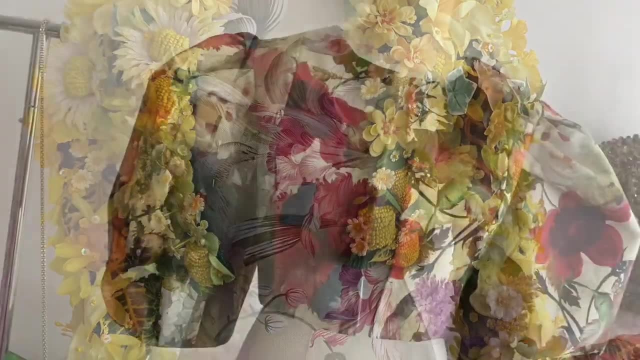 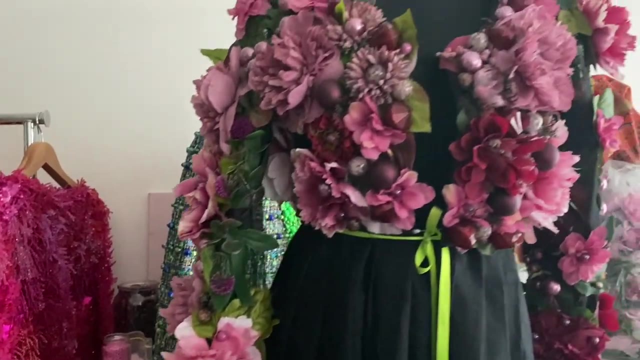 all the bags in the background and try and find a few more flowers so I can finally finish this. It's perfect, Perfect, perfect, perfect, Perfect jacket. I did say I was going to make a tweed jacket, but you know what Life got in the way. I yeah, the tweed's just a big piece of fabric. 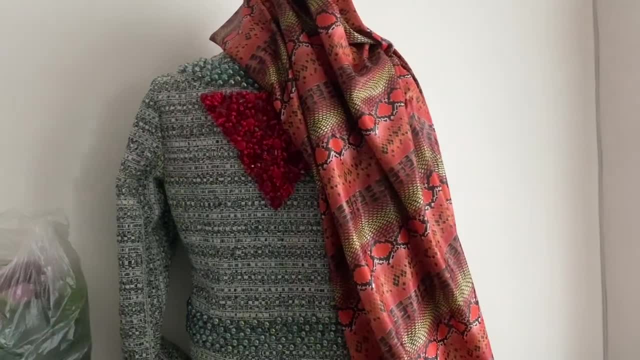 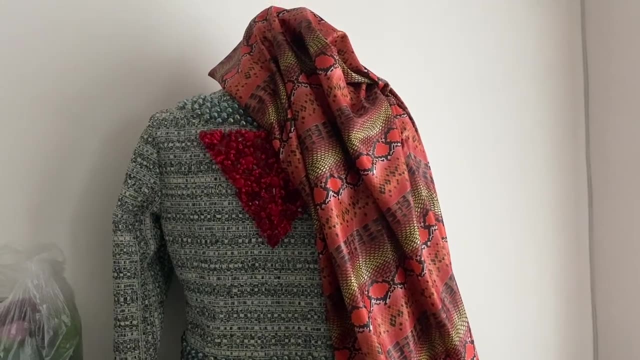 still, I have a few hours where I could have done some sewing and I have that fabulous snake skin fabric that I bought and I was like, oh, you know, I could, maybe, just if I work really, really hard, I could make a tweed jacket. I did say I was going to make a tweed jacket, but you know what, 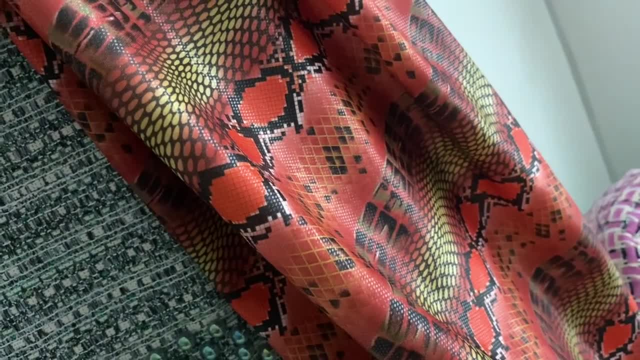 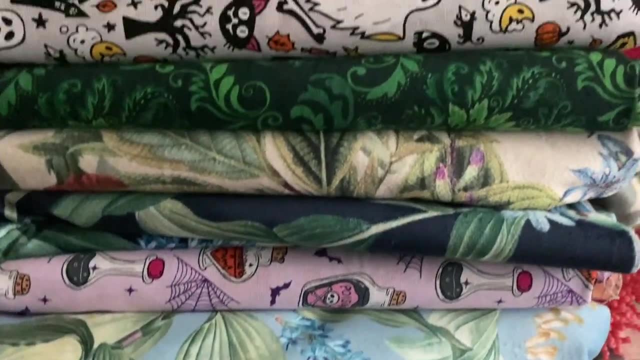 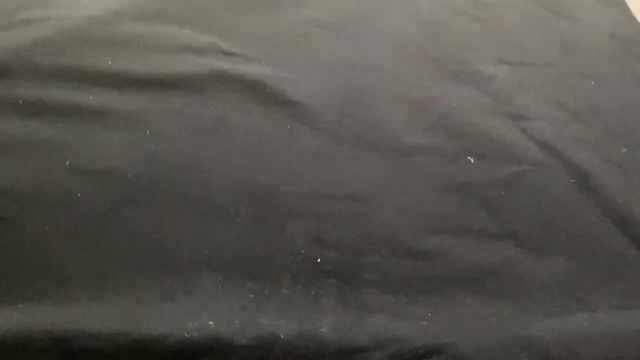 Fast. I could maybe make a jacket out of that, because you don't have to do as much hand stitching when you use a non-tweed fabric. obviously because it's not going to sag over time- It's basically just plastic- but I was like you know what? Maybe don't overwork yourself. So yes, these are some. 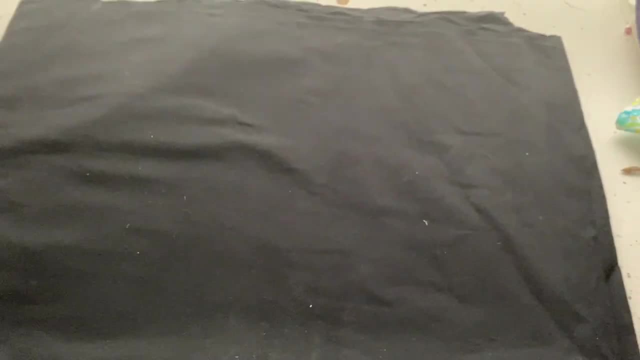 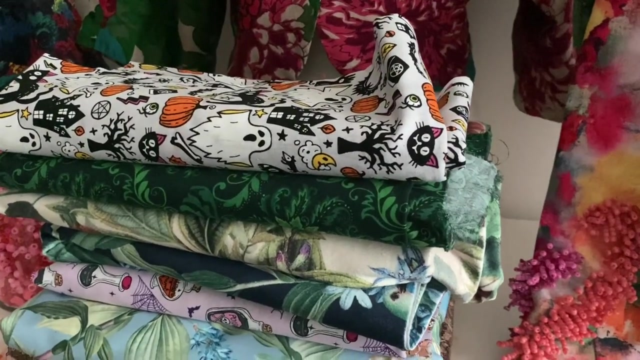 fabrics that you haven't seen before. This is just five yards of black fabric. I just put it down. Pretty exciting stuff. So here we go. We'll go with the colourful ones, So a couple of them are some of my favourite fabrics. I've got a couple of them. I've got a couple of them. I've got a. 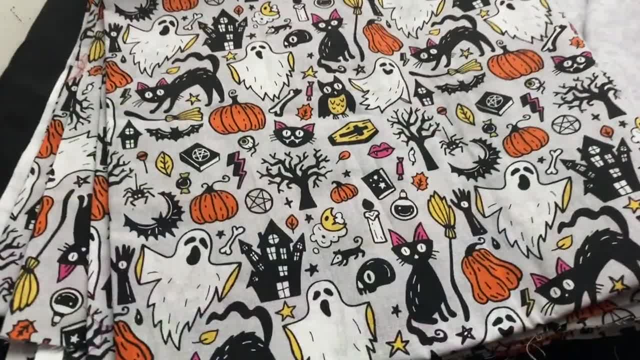 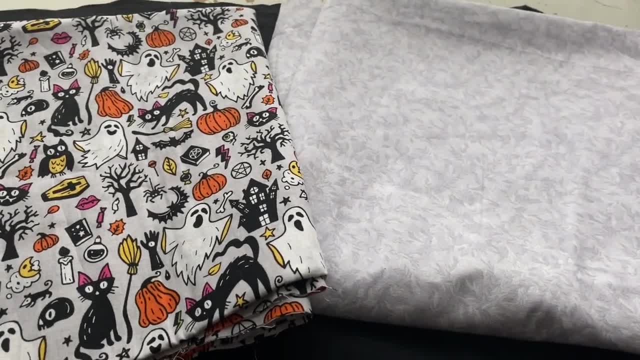 clearance fabrics, Halloween fabrics that you haven't seen before. This one's got a grey base and it's the cats that I fell in love with. on this one It's just got some weird stuff. So you've seen this pale grey fabric before. It's two yards of one, two yards of the other. 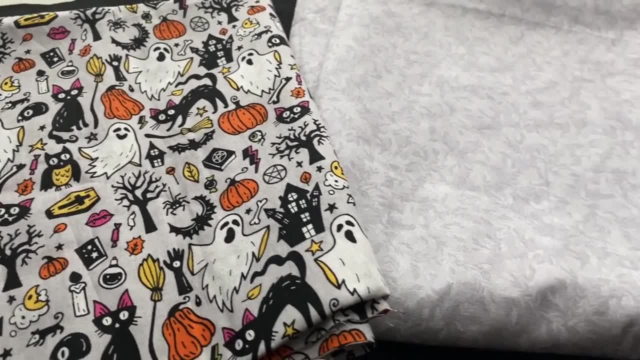 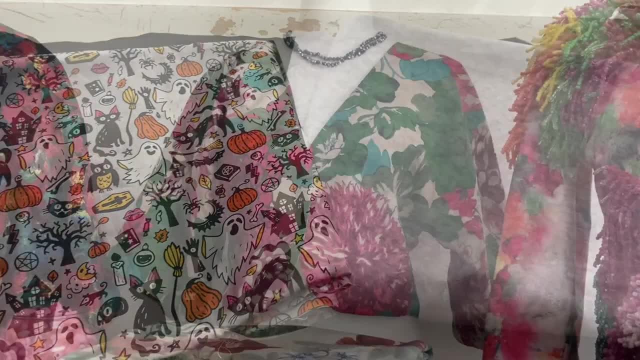 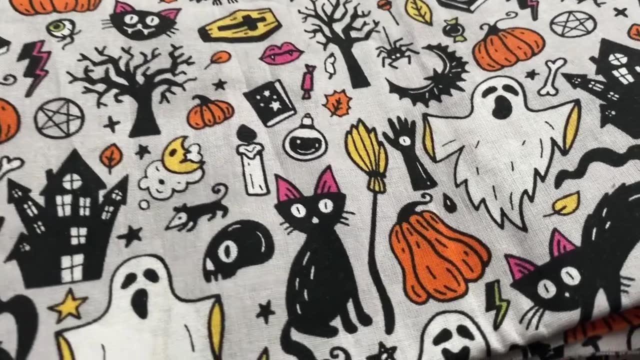 and I just thought that would make a nice dress. I've since bought this Liberty of London fabric, which is apricots and beige and cream and grey, and so, yeah, I think I'm going to make a jacket out of the pale grey one and the Liberty of London fabric like a reversible jacket. 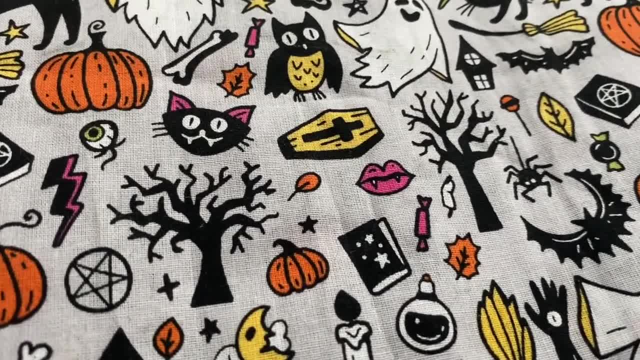 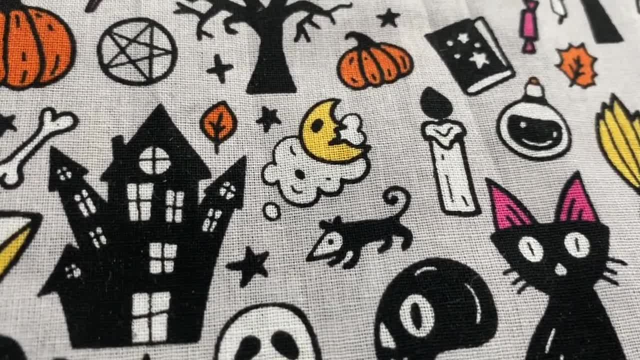 like the one I just showed you, and then with the remains of the fabric. So there'll probably be one yard of each of those and two yards of this. I'll make a summer dress out of that and I love the cat. It just looks so daft and I can't decide if that other animal is supposed to be like a. 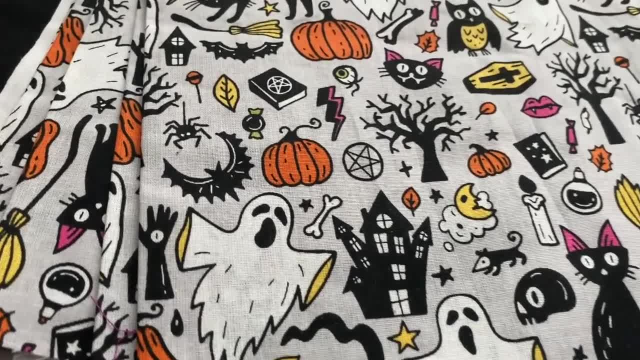 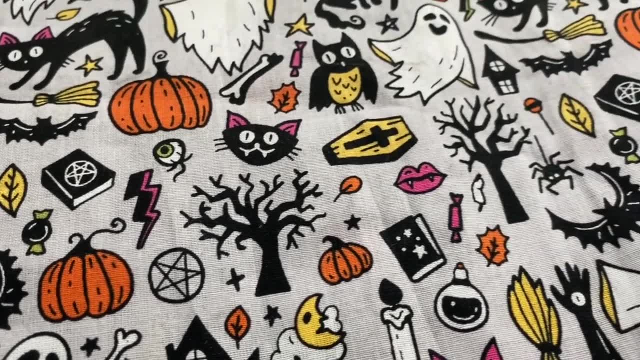 opossum or a dog, or there's a bone. So that's why I think maybe it's a dog. But the bats, they're all just a little bit weird. but the cats, I just thought they were so cute. Yeah, it's just a bit random. It's like they had little gaps in there and they're like 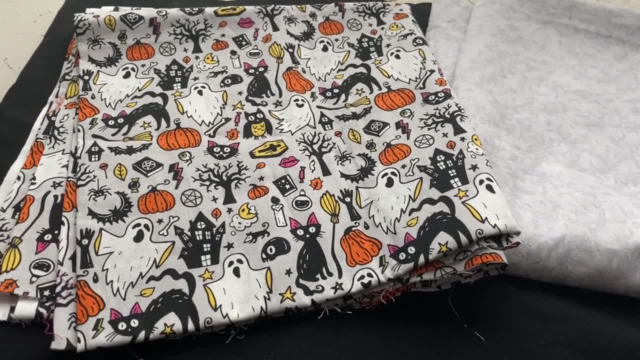 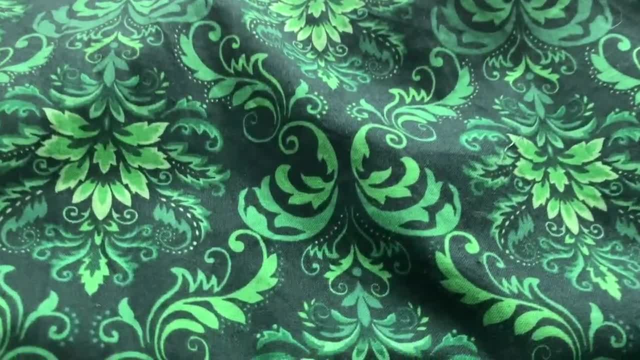 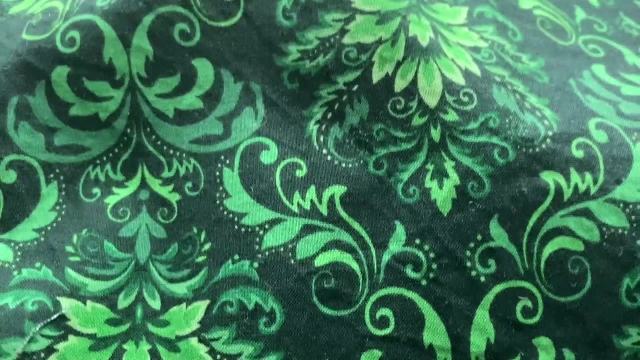 oh, and we'll put an autumn leaf here and a bit of candy here, and some loops here and a weird cartoon skull, Anyway. so the next fabric is another quilting cotton. and yeah, I've washed this, but I haven't ironed it yet, So I just thought it was beautiful. It's when you 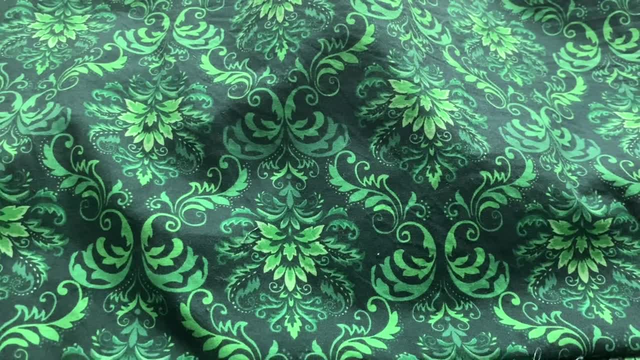 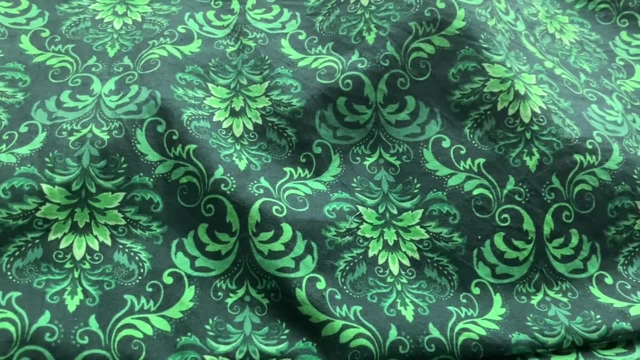 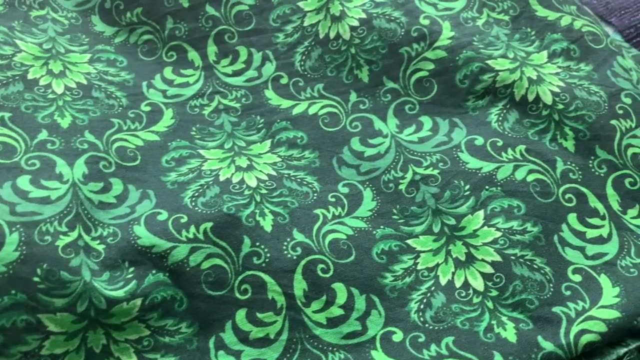 it's just one green on black, but it's actually lots of different greens and that's what I love about it, I think. So I've got lots of green beads, obviously because I love green and I just, you know, it's the colour of nature and I just think this is beautiful fabric and 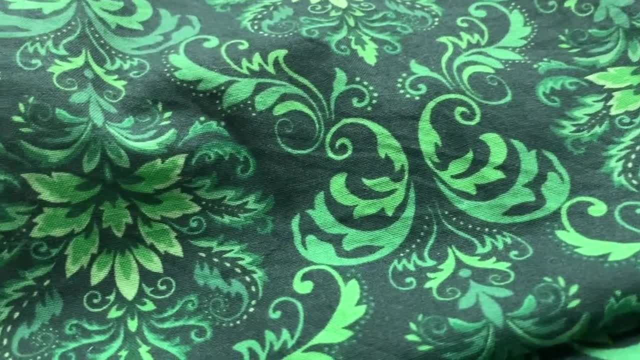 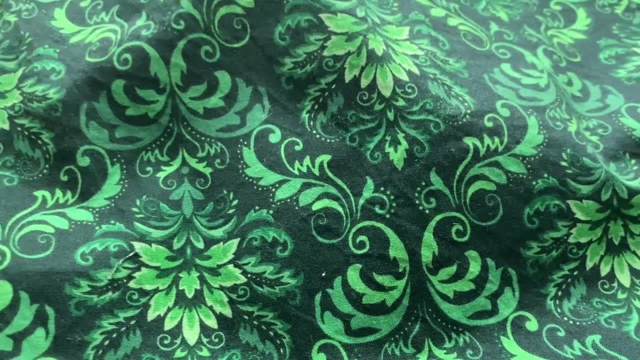 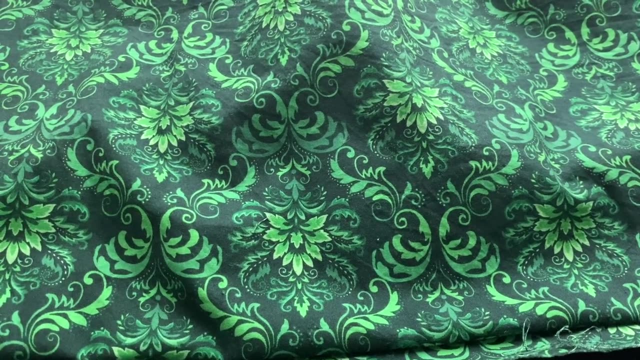 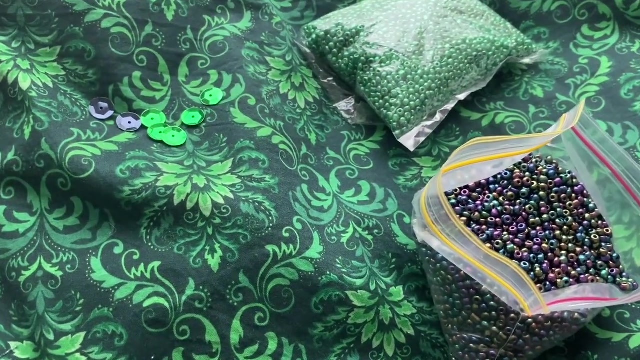 like when I first started making jackets. I made this one out of a quilting cotton and it's sort of on it and it's William Morris, but I bought it like a decade or maybe even 15 years ago now and I turned that into a jacket and then I beaded over it with green bugle beads- metallic green bugle. 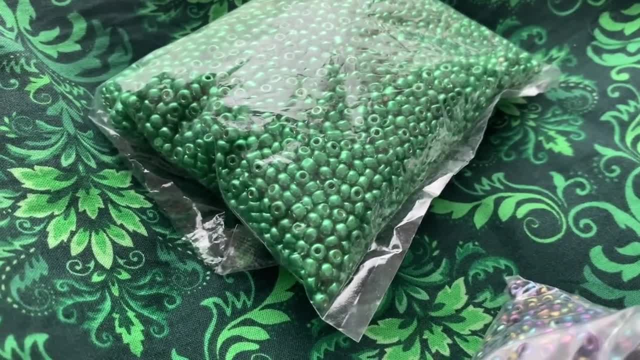 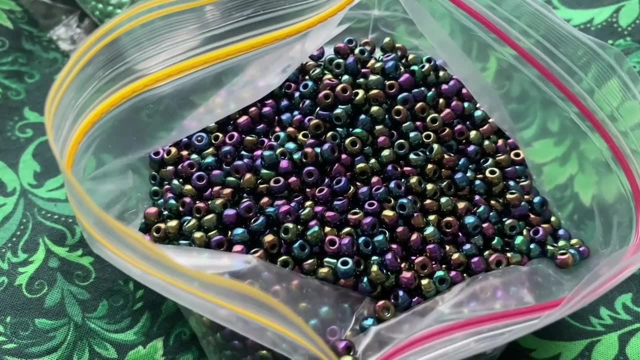 beads and I love it, but I would like another one, that's, you know, same but different sort of thing. These are black beads with iris. that sort of metallic sheen on them in different colours is called an iris finish and they just, you know, they're just sort of like a little bit of a 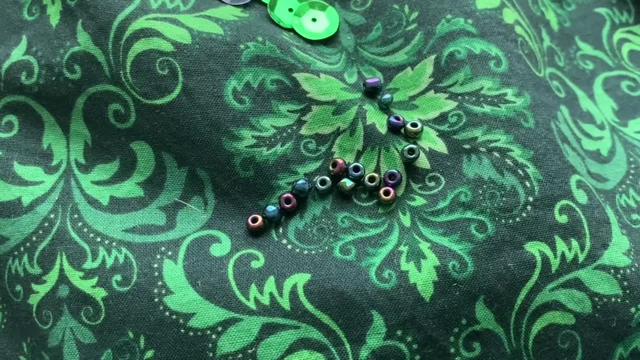 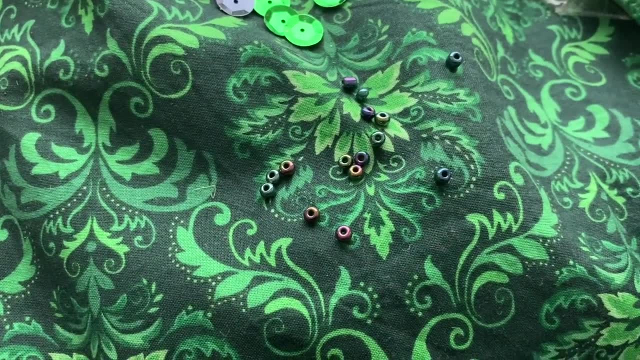 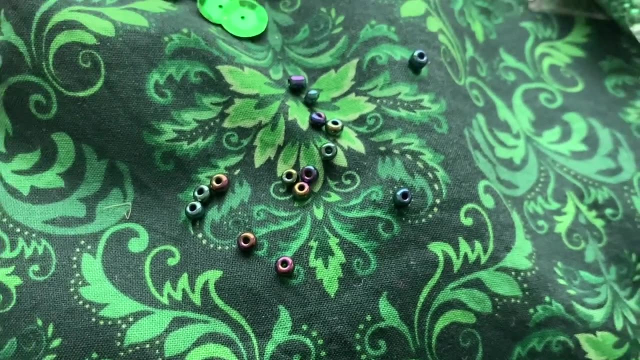 look absolutely beautiful, like obviously, when they're stitched on they're going to sit up right and yeah. so I'm thinking of just making the jacket out of the quilting cotton with black tulle over the top so it sort of mutes the quilting design a little bit, and then I'm going 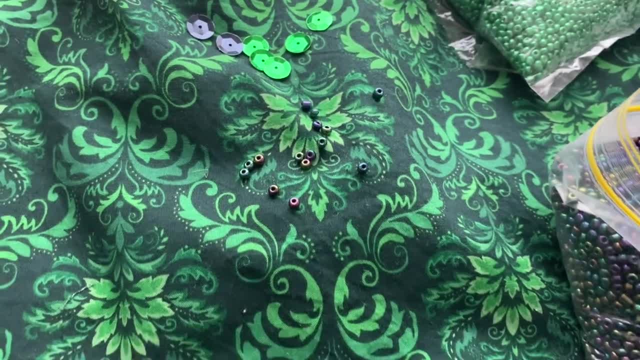 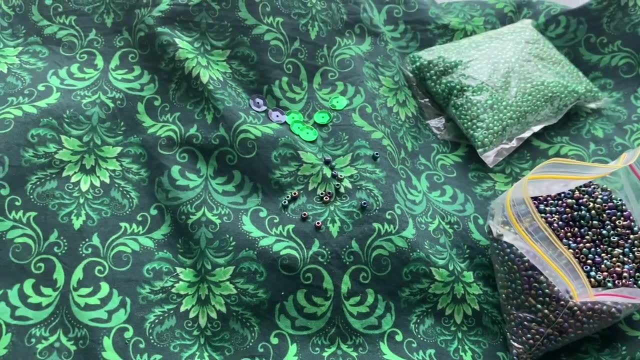 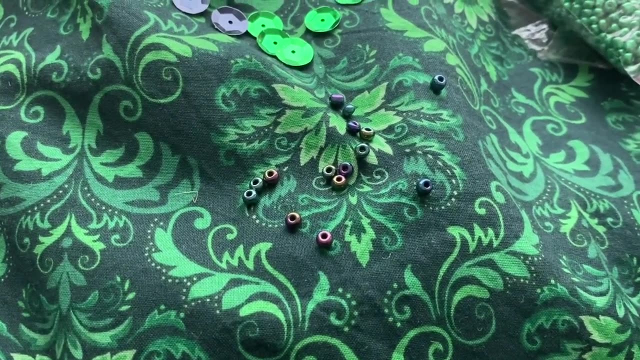 to hand stitch all these beads on over the top to sort of bring out different aspects of the. I mean I've also got out some sequins. I've got like thousands of green and black sequins in this mix. they're like leaf shape, flower shape and then some. 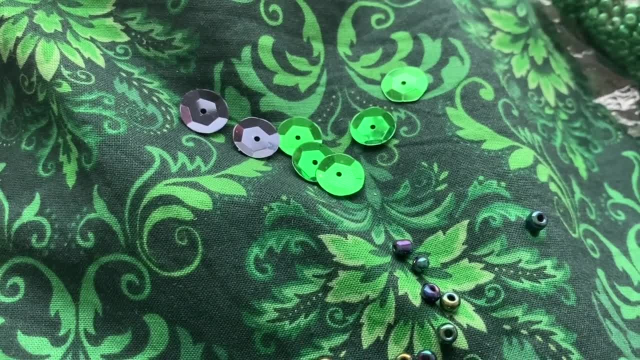 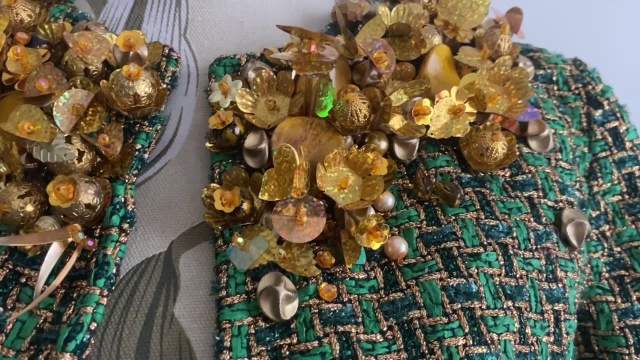 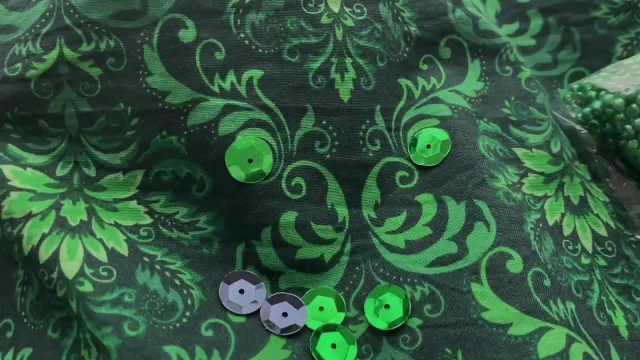 vintage ones in there as well. so I could do that, like collar and cuff beading or, you know, highlight different aspects of the pattern, the motifs in the design. but I don't know, I think maybe I'll go with the small, the seed beads in the black, and I've got a couple of 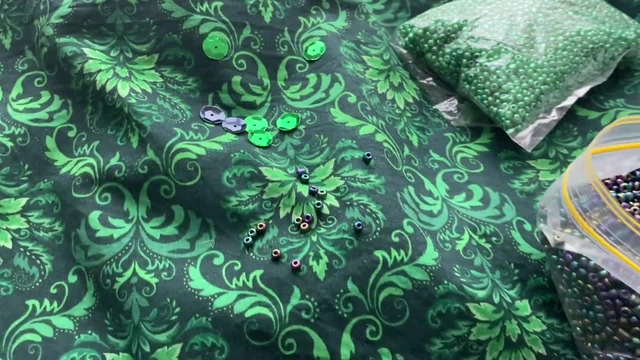 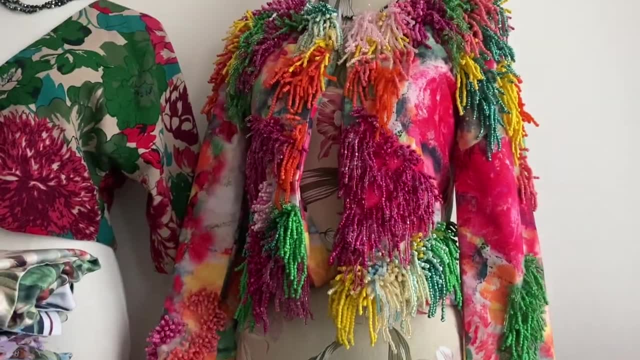 different greens, like a metallic green and then just a solid and a frosted green glass. I don't know. I just know that I want, like a summer weight jacket in those sort of colours and yeah, so I've put it under that jacket because that's the 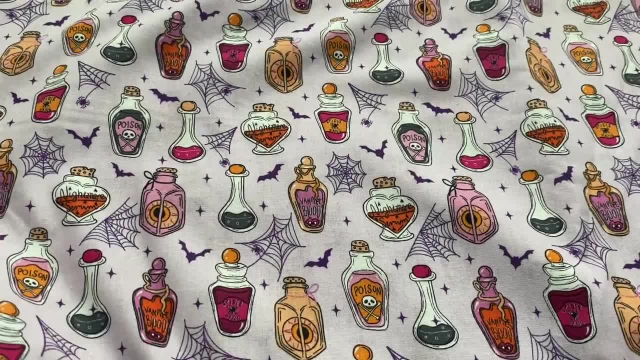 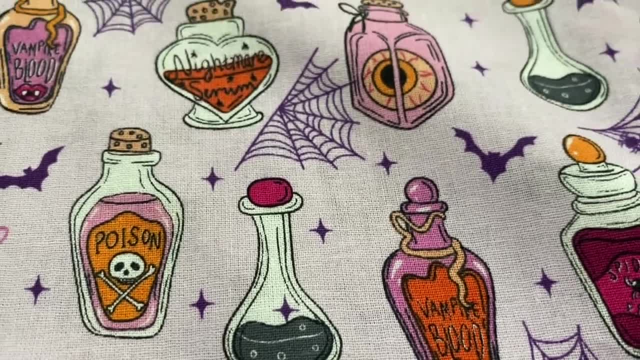 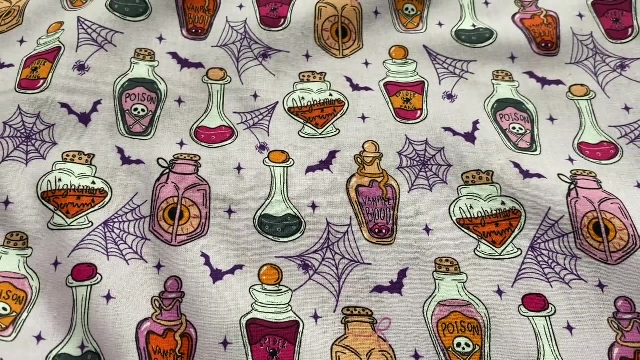 jacket pattern I'm going to use, and this is the second Halloween fabric. I just love the colours. it's kind of a I love that mauvey pink colour. it's absolutely gorgeous. I've got a jacket that colour and yeah, so I was going to. 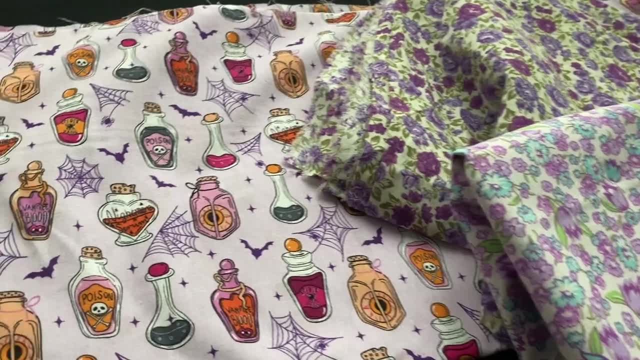 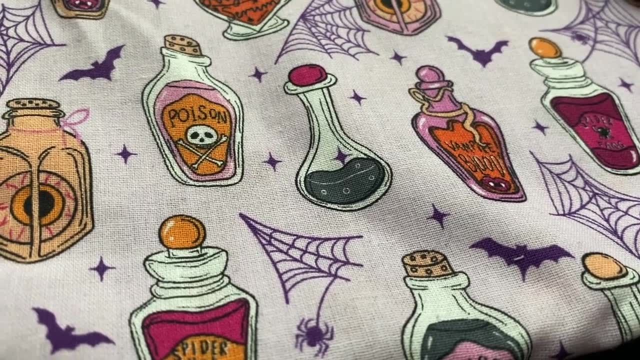 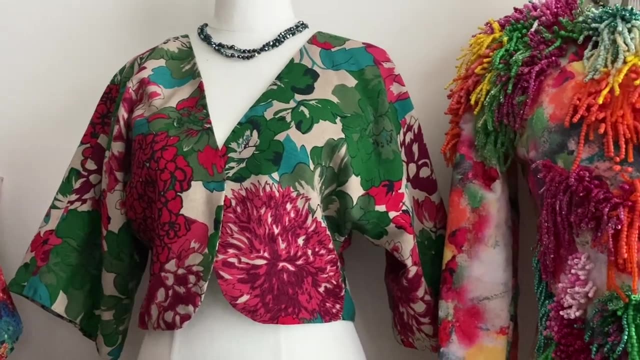 make a dress out of again. I was going to make a few cotton summer jackets, reversible ones, and out of the floral ones. so and then, like, one side will be the this love potion or different potions one. I bought this, yeah, so it'll be two different sides. I'll probably wear the floral. 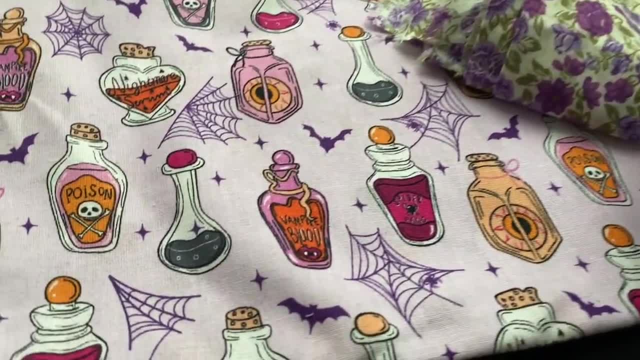 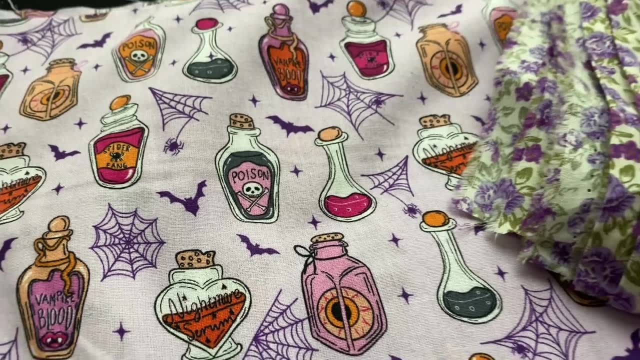 side most of the time, but it'd be cute to have this on the cuffs that you turn up. I bought this because it reminds me of you know that movie, The Emperor's New Groove, where the bad guy is Esme, and she's got that. 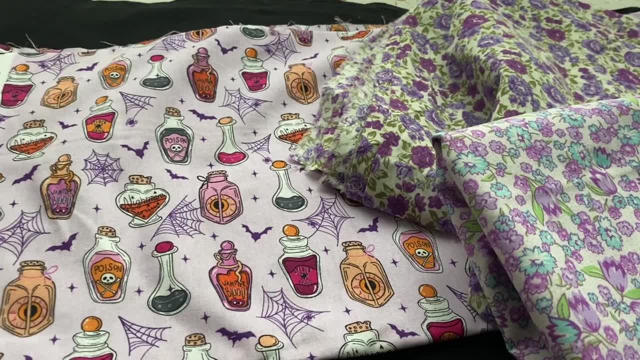 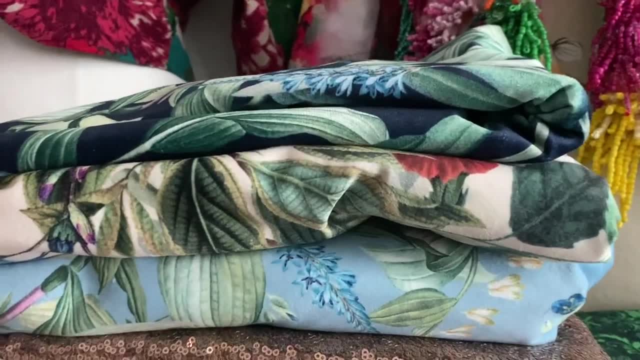 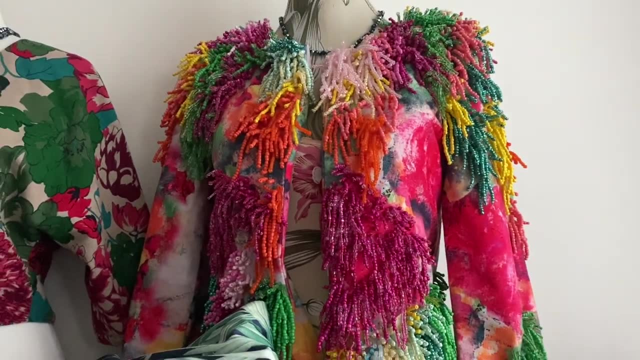 underground lair and she's got all those potions. I love that movie. it's just so silly and in just the cutest way. Anyway, the next fabrics. oh, I think we have three home decorating fabrics. they're like velvets, the same as the Kandinsky's home decorating velvet. that's like a really tough. 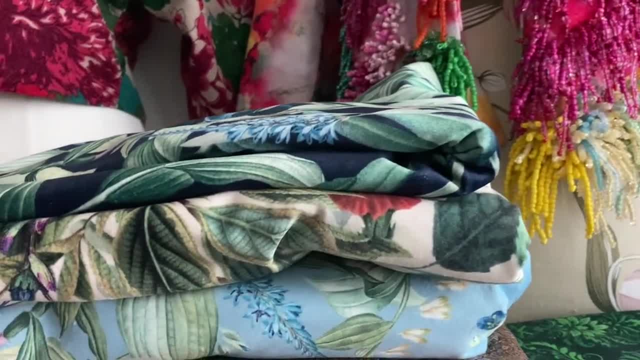 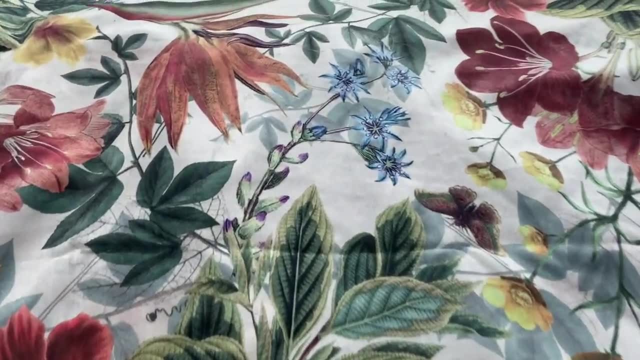 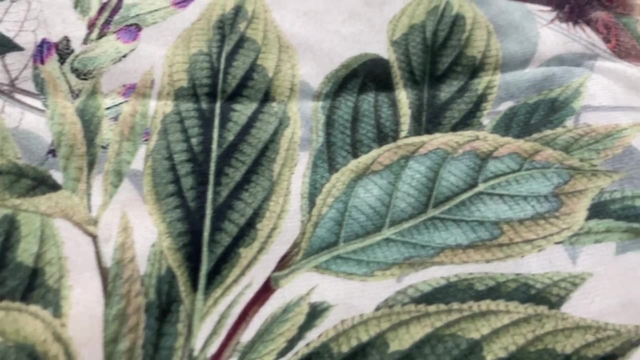 sturdy velvet And they're just really really good to bead into. like that has so much weight in beads on it. So I showed you this one in December. it's the one with the birds of paradise and, like, I just love birds of paradise but because I'm such a small stature of a person, I mean I can't use. 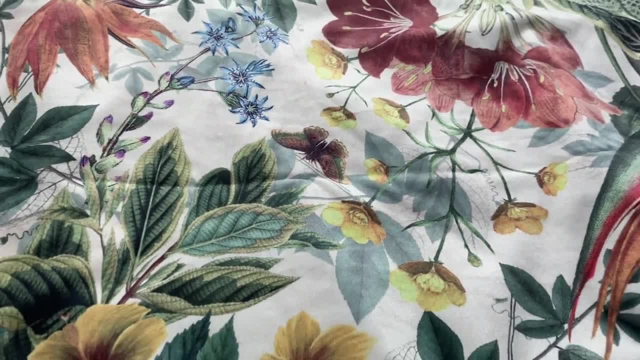 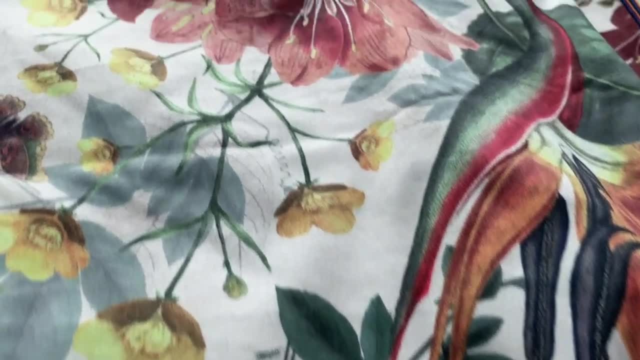 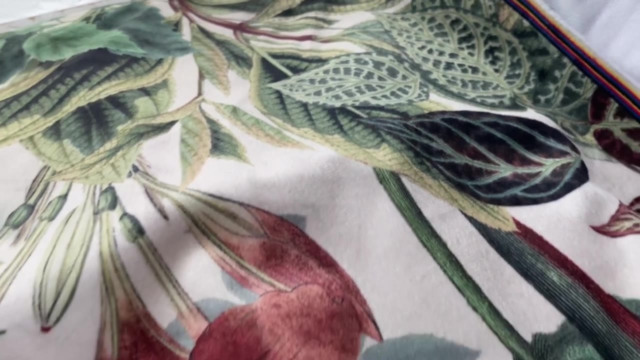 them on my floral jackets or anything like that. but when I saw this fabric I was like, oh my gosh, I can make something like I can make it like that Kandinsky jacket out of this one and I was like I can do normal beading on it. but yeah, I've, since I love these leaves too, I think I'm a. 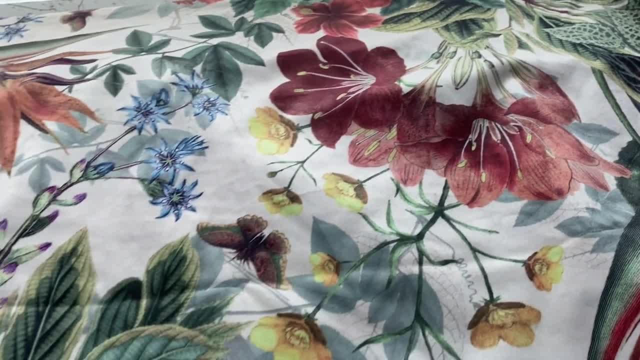 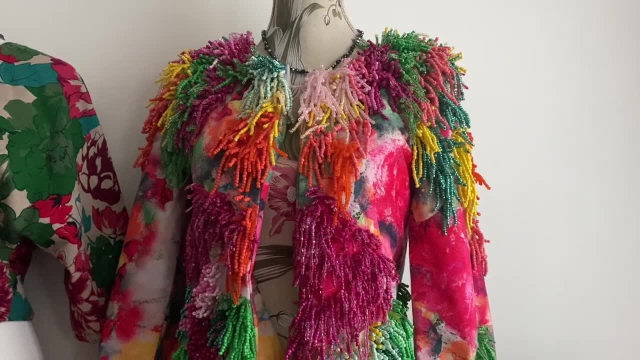 sucker for a beautiful variegated leaf, Anyway. so yeah, I was going to make a jacket out of this and just bead it using my normal size beads, but now that I've done the Kandinsky one, I think, I think I'm going to do the bird of. 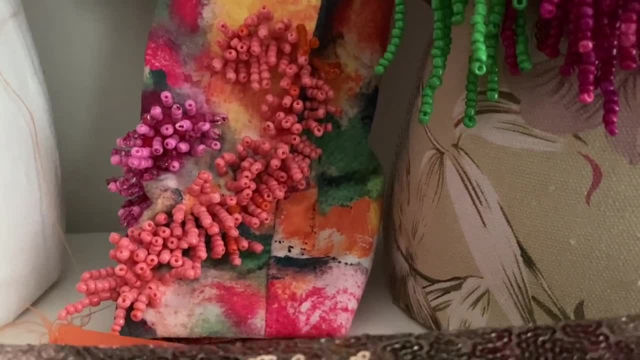 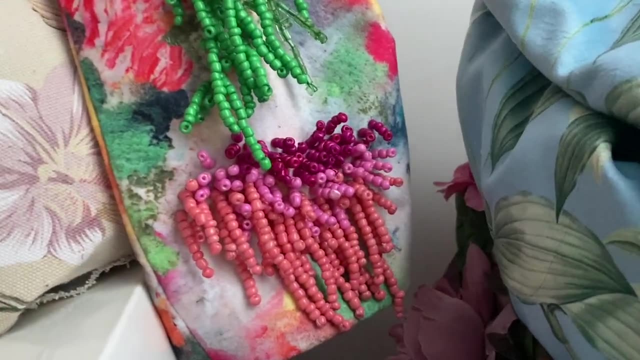 paradise one. See these ones here, how they're sort of much shorter than the big strings of beads. well, yeah, I think I'm going to do that, I'm going to do that, I'm going to do that, I'm going to do. and there's more of these on the other cuff too. see how it's like short, short and 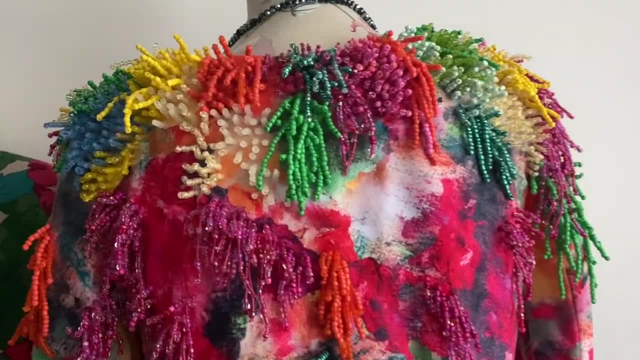 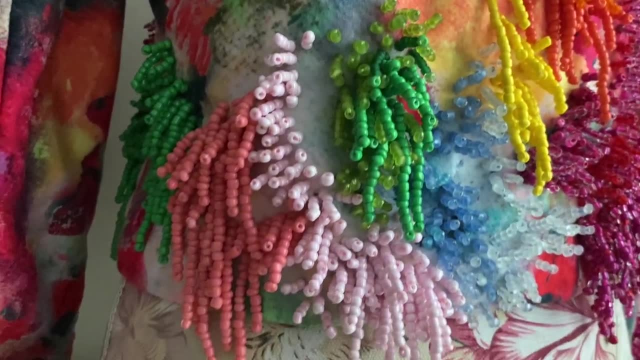 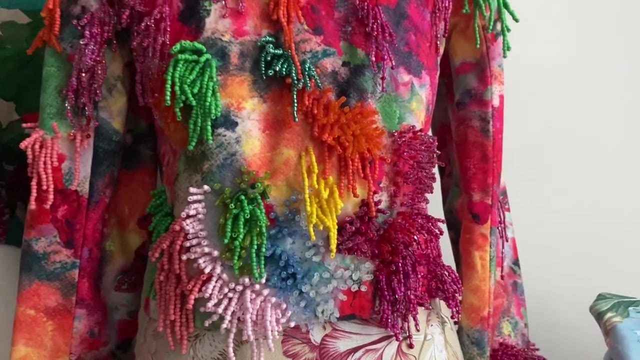 then longer ones and then on the back too, it's a real mix of short and long. I like this, like I love the front of this one, but weight wise it is quite the heavy jacket. So I think I love the mix of like different heights and it just makes it look so much more. 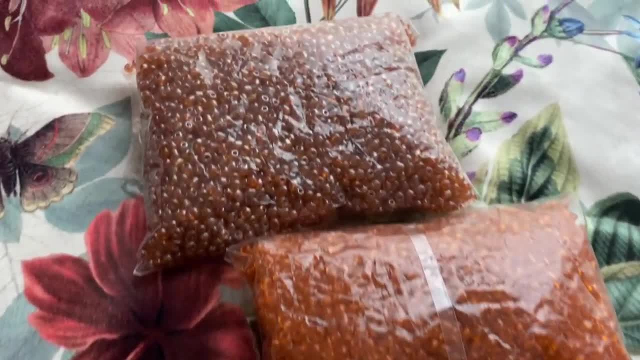 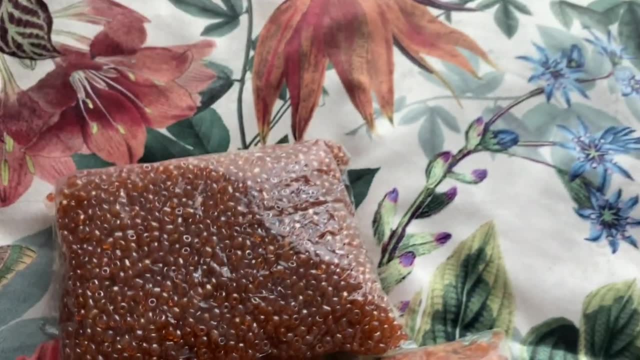 textural. So, yeah, what I'm going to do on this one is I've got some autumn colored beads and I just bought them because I've got an autumn harvest floral jacket that I'm going to make and you need beads to stitch things on. 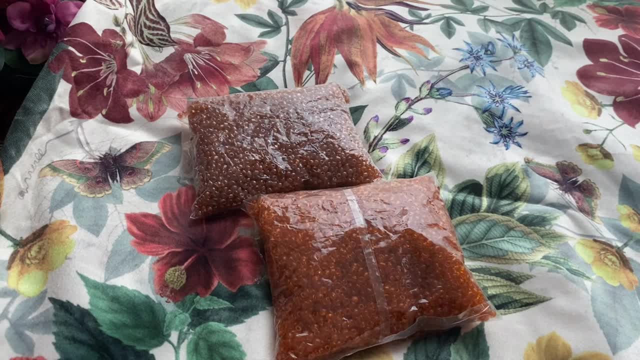 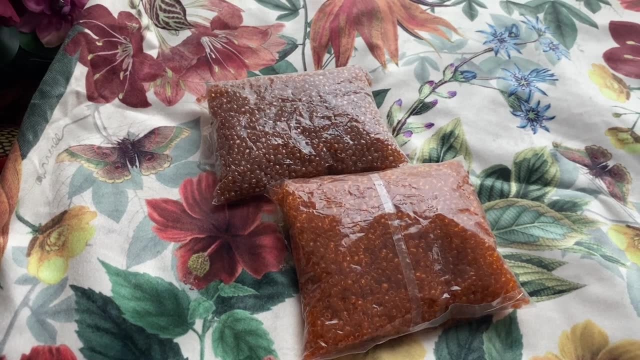 So that's why I bought these beads. So there's going to be about half of them left over anyway And I thought maybe I can use them on this. Like, the background of this is a sort of creamy color, and I do have lemon, cream and beige beads. 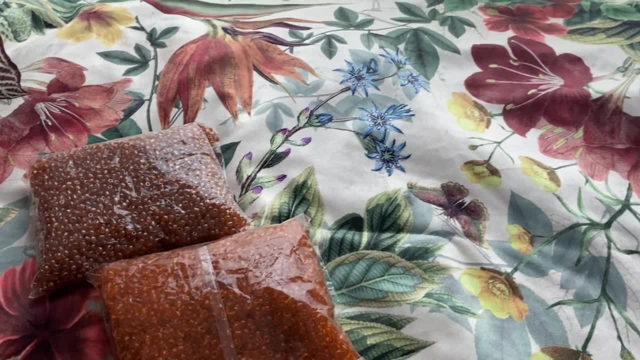 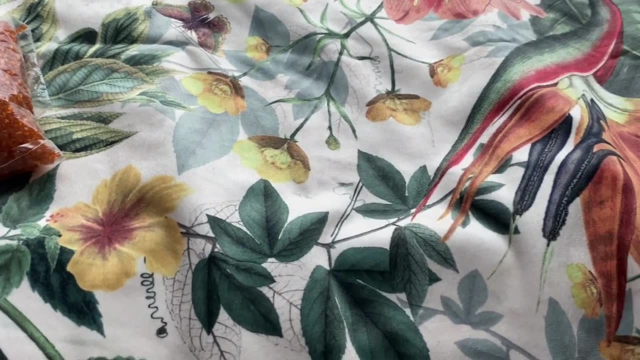 but I just think it would be amazing if I over beaded it all and darkened the entire entire jacket down to the same colors as the big flowers and the bird of paradise and sort of just left the merest art line around the flowers. 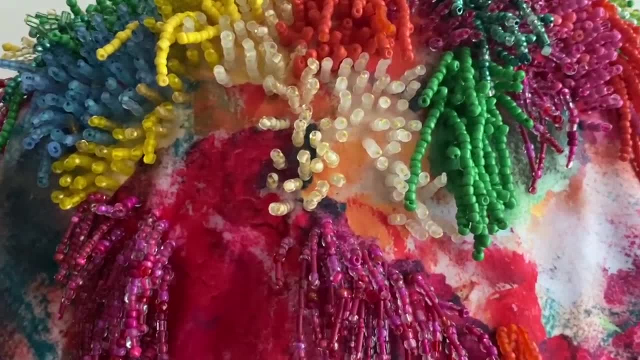 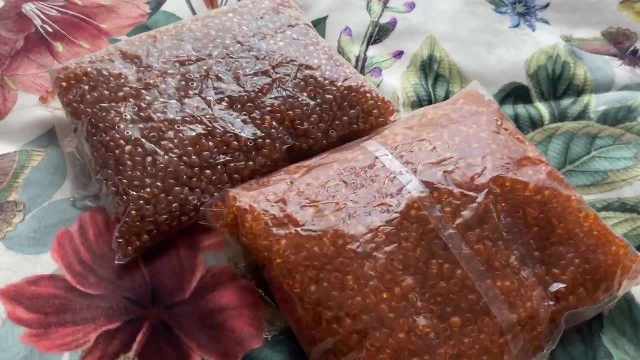 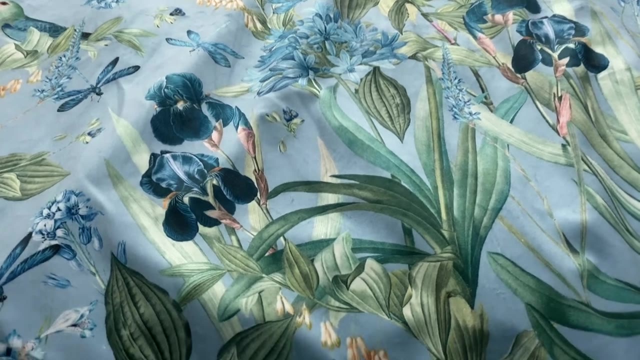 And most of the jacket was just this really dark, like cloud configuration of different autumn oranges, burnt oranges. I know what I mean And yeah, so that's what that's my thinking for that one, And then I have two others. 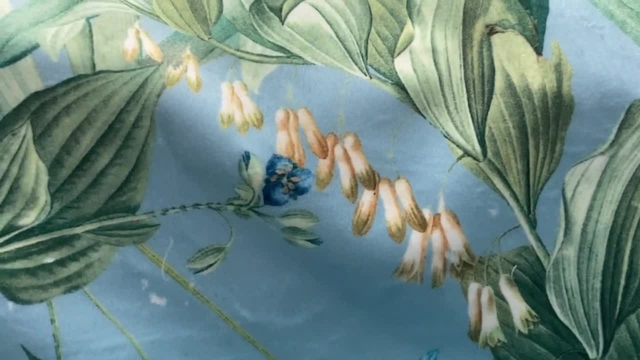 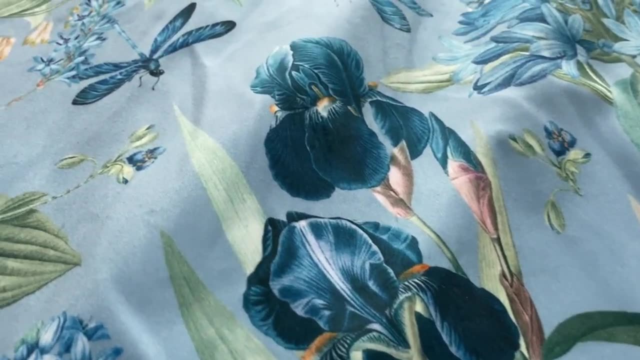 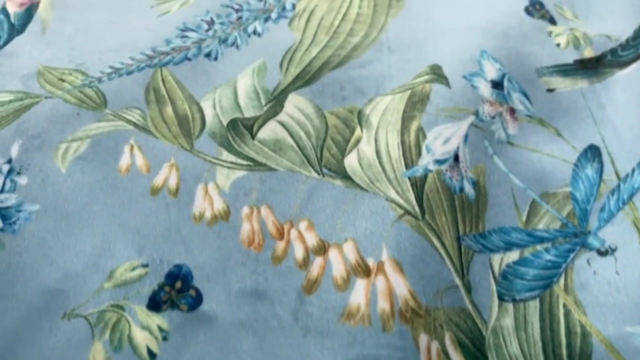 I actually have this. It's in two different colorways, So I just thought. those little bell shaped flowers always remind me of Tiffany, stained glass, and the iris are beautiful. I love everything about this- The dragonflies- and there's also a bird in here and some other little flowers and I don't know. 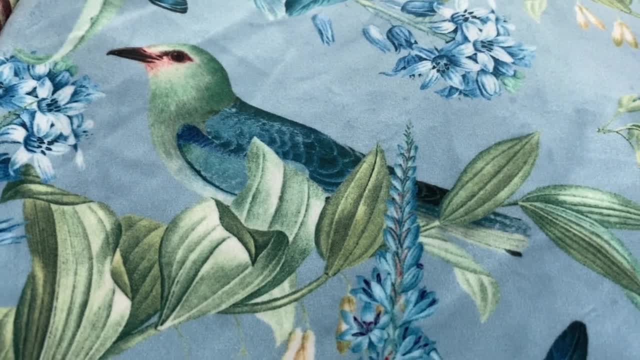 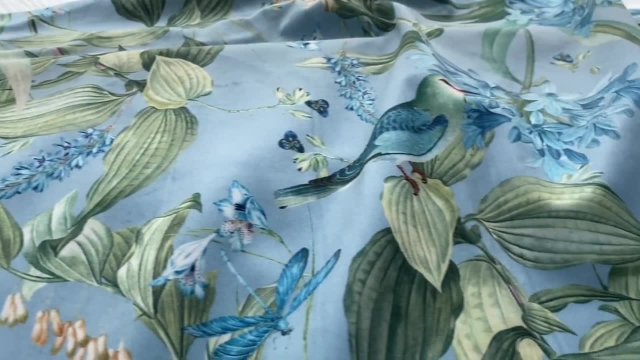 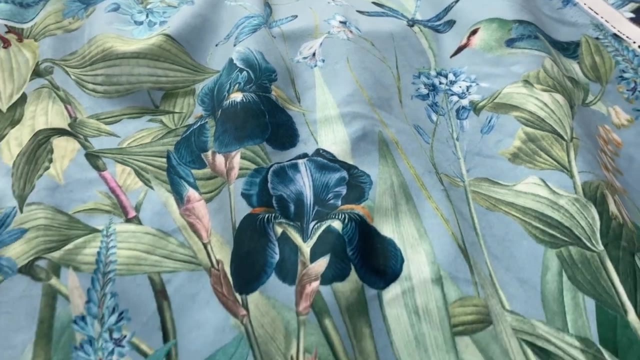 it's just so pretty. See this bird and I love the peach of its beacon eyes sort of bit and the way that sort of goes in with the brown bits That are on the iris and the sort of orangey golden of those little bell shaped flowers. 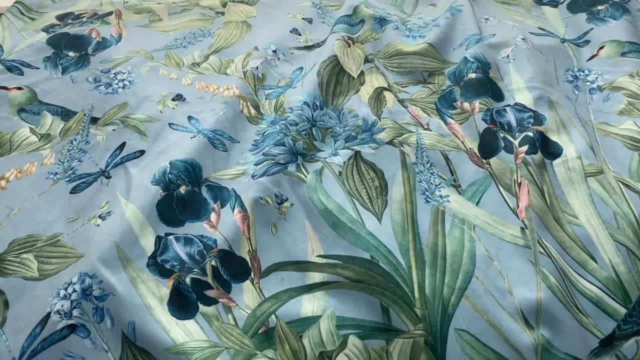 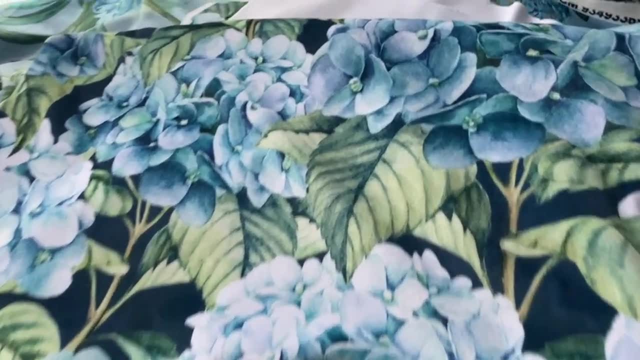 I just think it's. it's just so harmonious and there's so much detail in there. The more you look at it, the more you see, And I do. if it looks familiar, it's because I do have that, as you can see. 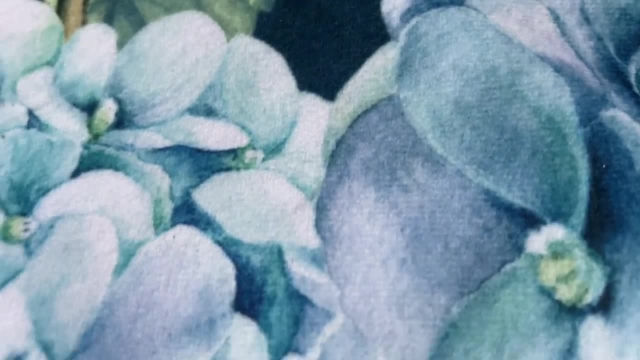 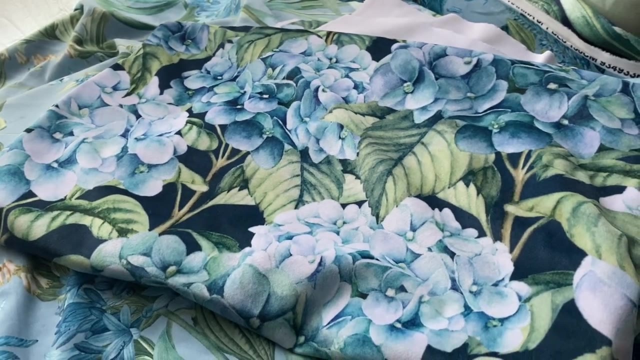 like the back is just it's synthetic, but yeah, And the front is fluffy, velvet. I'm not sure the velvetness of the fabric comes comes off particularly well in footage, but in real life it just feels beautiful and soft and velvety. 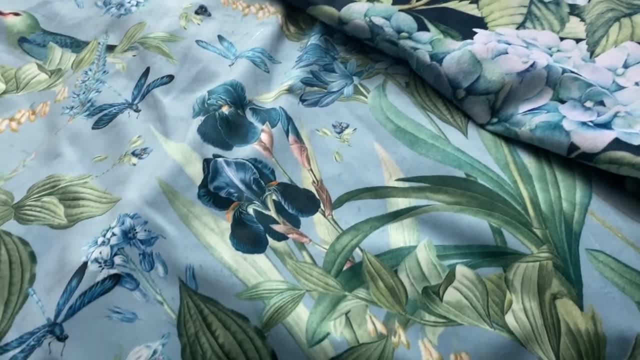 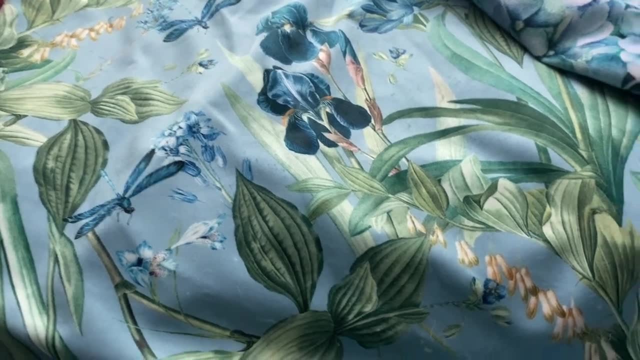 but it's also really sturdy So I can really bead a lot into it. So the hydrangea one is the one that I'm going to do in blues and greens and all dripping down The beading is kind of going to be like the Kandinsky jacket. 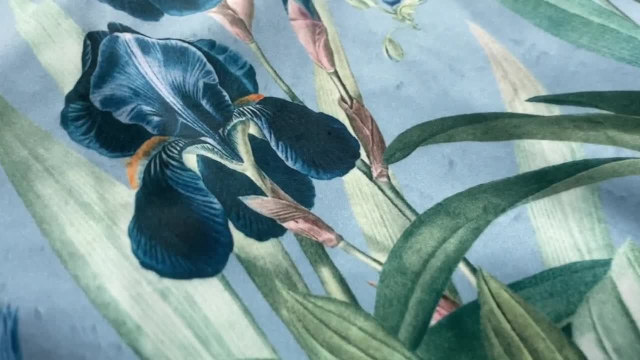 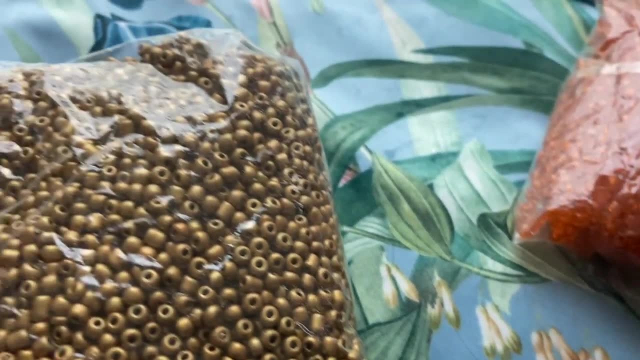 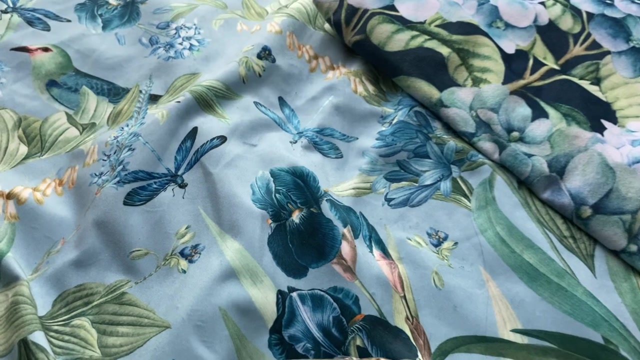 Whereas this one, I don't know. I mean I could highlight the gold and orange of the little bell shaped flowers. you know, just put a little bead here and there and then big strings of green um the, because the leaves sort of hang down on those ones, and then bead around, the dragon flies or something. 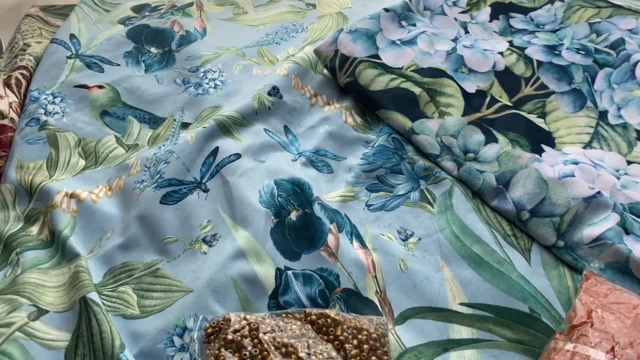 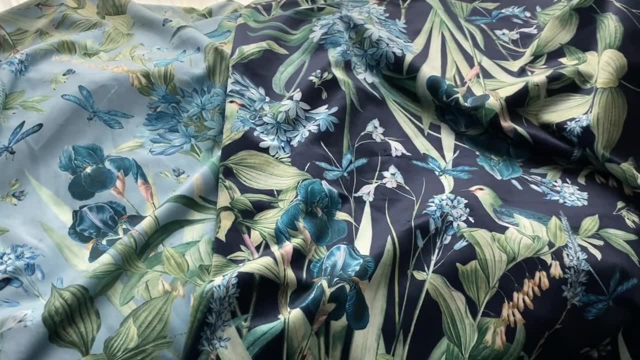 I'm not sure I'm going to make it up because the there's so much going on in the in the pattern, but it's also a bit epic, So it will really like if you have an iris on one side and then the dragon flies and the 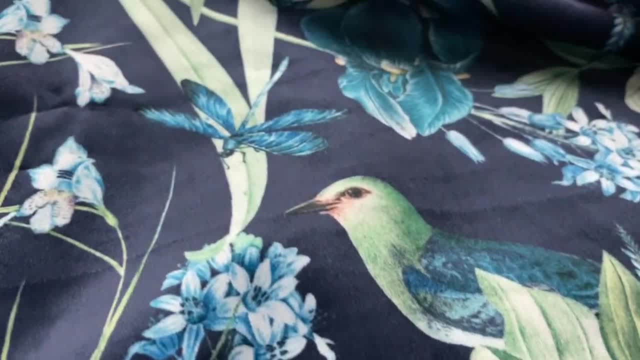 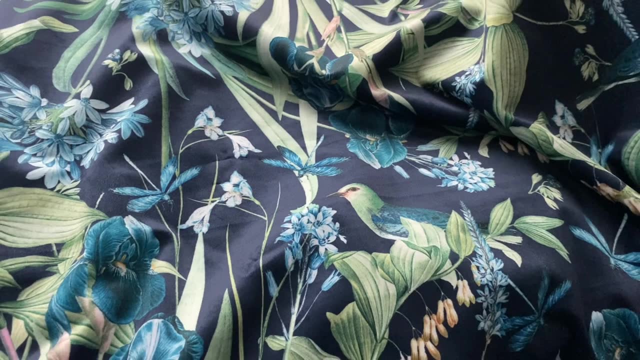 um, yeah, it sort of depends on the placement It will be, depending on how I end up beading it. And then, yeah, as I said, I got it in two colorways because navy blue? I always wear my navy blue jackets pretty much more than any other jackets because they just go so well. 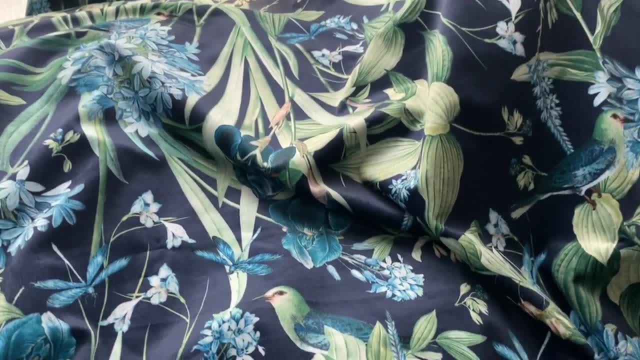 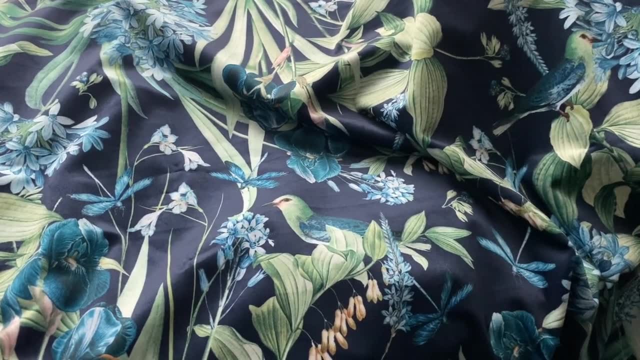 And it's really hard to see, like people who are they don't know what they're looking at. They just sort of go: oh yeah, navy blue jacket, And so you don't get much attention when you're wearing a navy blue jacket. 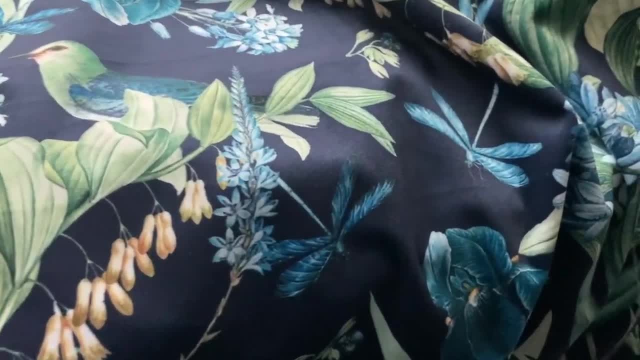 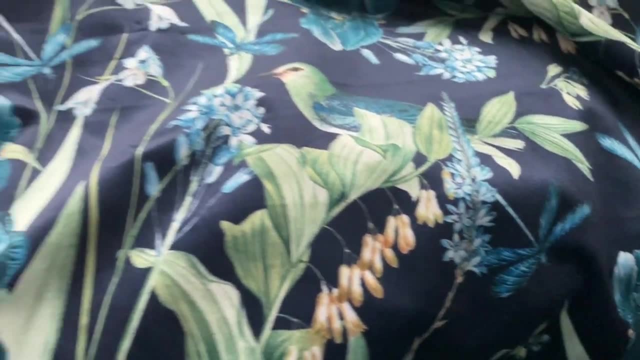 So I quite like them for that reason as well, But, um, I just think they're beautiful too. So, yeah, Um, what I like about this one is different aspects of the design really stand out, Like you can see those little bell shaped flowers, and they look much more golden and orange in this one. 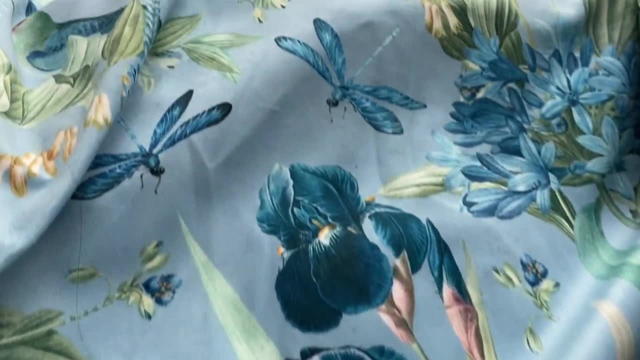 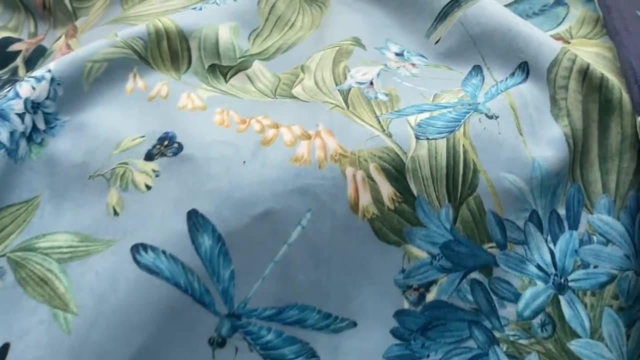 whereas they almost fade a little bit to the background of here, Whereas the dark blue iris are quite clear and the dragon flies, kind of. they just look completely different in the two different versions of the exact same design, But because the coloring is different. 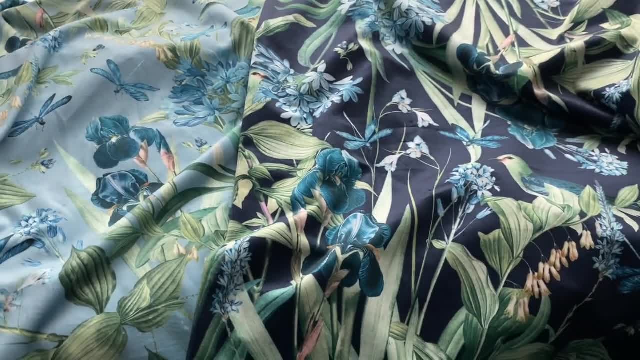 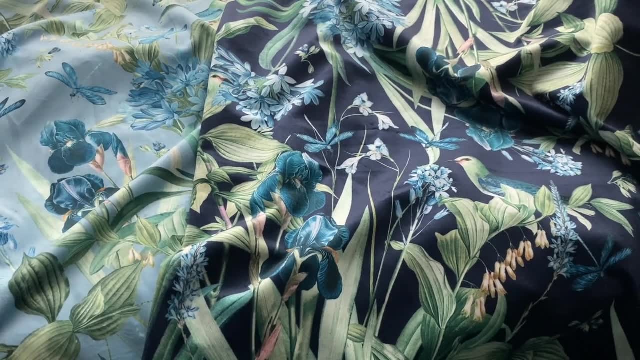 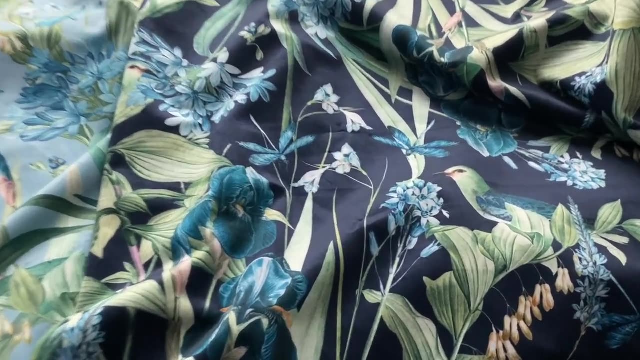 different things stand out, like the. I feel like in the dark one the bird kind of almost sinks entirely into the background, Whereas in the light one you can see it more. I don't know, I just like both of them and I want to make them both up into jackets, and then I'll decide how to be them. 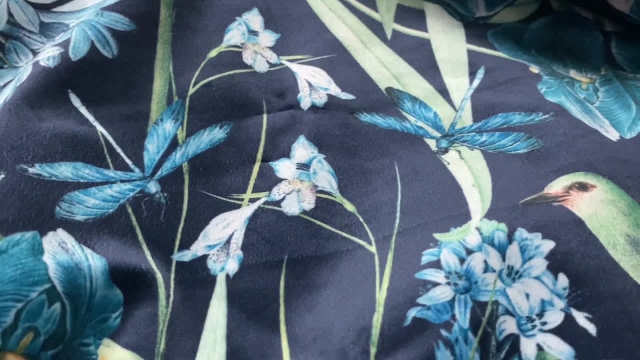 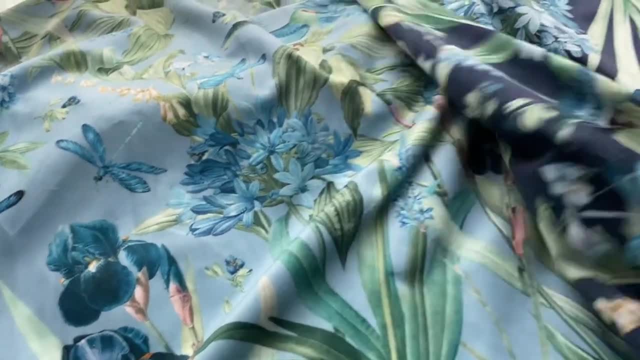 Cause I do have um a lot of dark green and dark blue beads, uh, glass beads, So I mean I've got, I've got, I've definitely got enough beads to this is me trying to find the two birds so you can compare the birds of each. 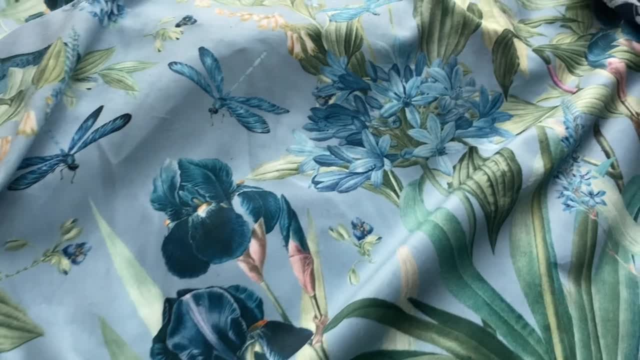 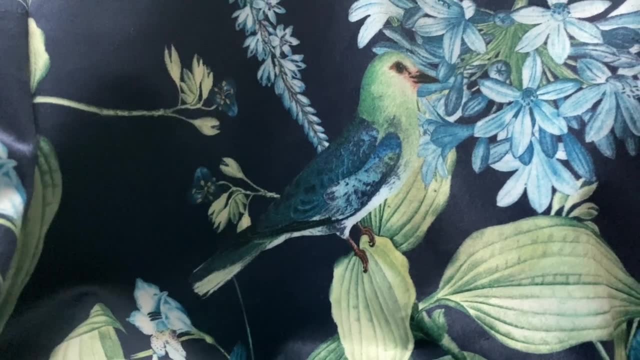 I think. But yeah, they're just absolutely gorgeous And of course they're both velvety, so they feel beautiful. I love this bird, but I do think it sort of um goes into the background quite a bit, Whereas the other one 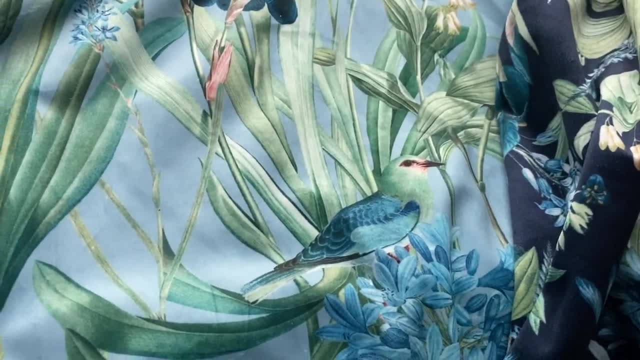 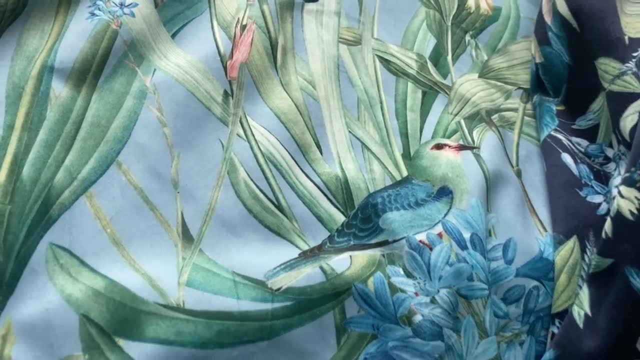 I don't know, especially if you put like green, um bit seed beads in on the um leaves behind it, Of the bulb plant behind it, it would bring out the whole of the bird Like see, if you beat it all this bit here. 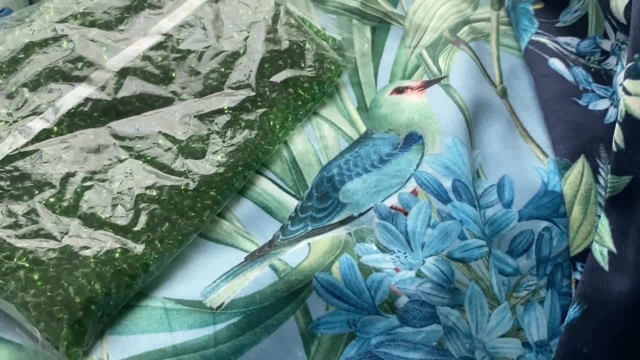 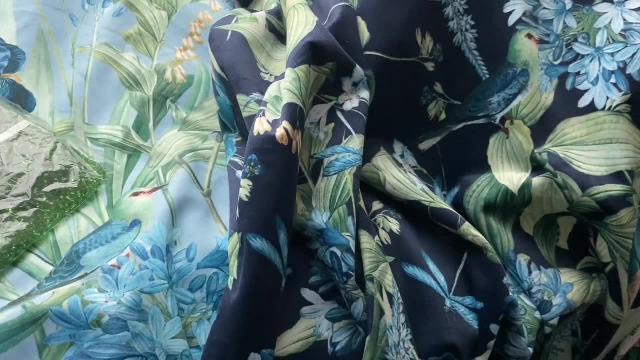 I know it sounds like it wouldn't, but it will actually bring out the bird and it'll push back the rest of the background. So I kind of have a few different ideas for it. but yeah, it really depends which part you highlight on. 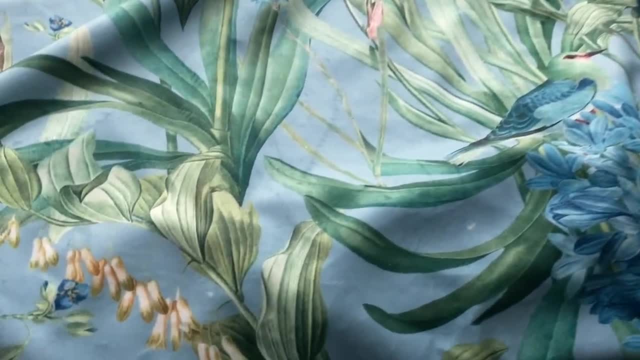 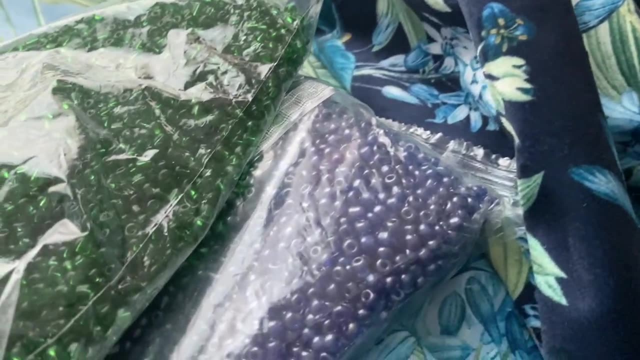 You know, I w, I think I want the iris on one side, um, on the other side, on one side of the front, and a bird on the other side of the front and then maybe some dragonflies and iris on the center of the back. 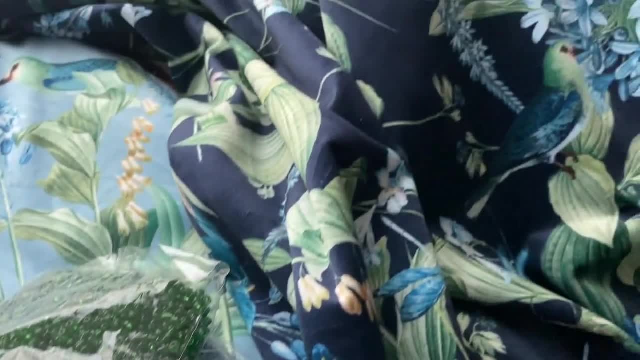 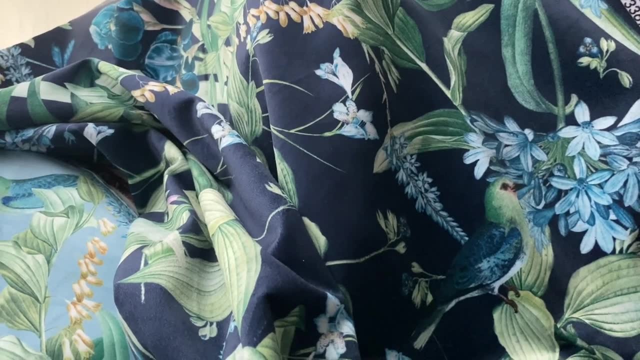 And then I'll sort of do make features of each of those bits and sort of bead out some bits so that they blend into the background and bring back up other bits. So yeah, I've got lots of beads, so we'll see how that goes. 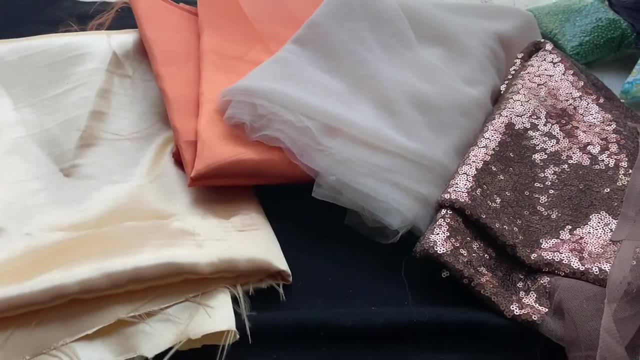 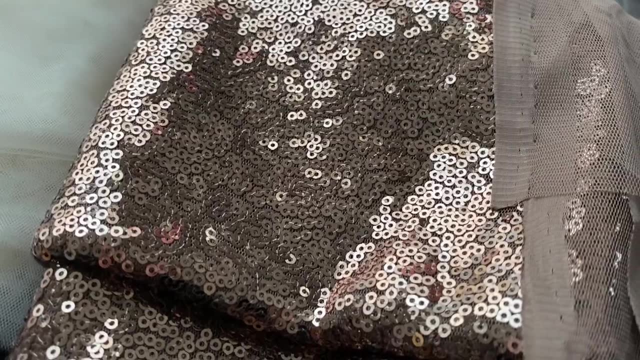 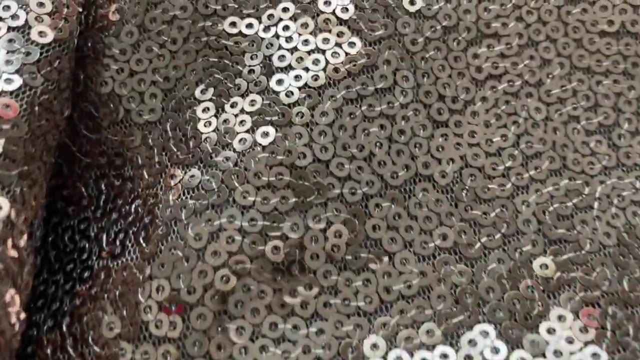 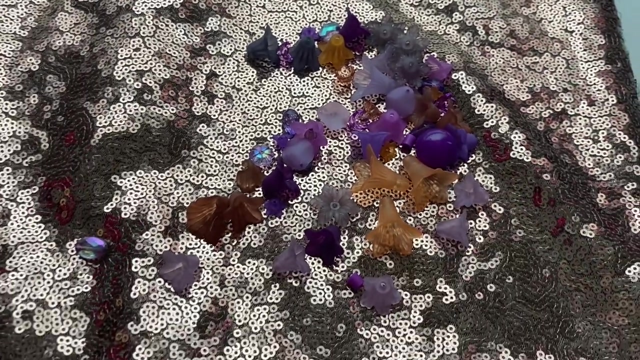 And then we have four fabrics left. This one here is a brown sequin fabric. I've shown you a very similar one, but yeah, I'm just going to. I had one that's pretty much exactly like this. It's just slightly different color, and I'm going to put brown and purple flowers beads on that one. 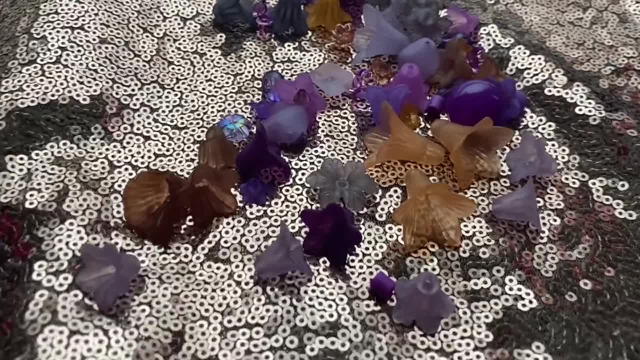 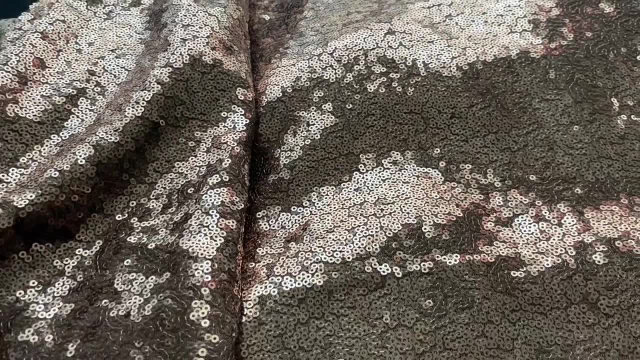 But I also have a lot of brown beads and gold beads, So that's why I bought that one, Cause I had. when I had the one bit of sequin fabric I was like, Oh, do I do the beads Or do the flower beads? 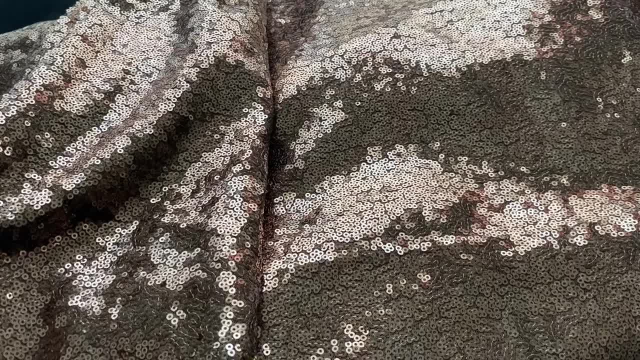 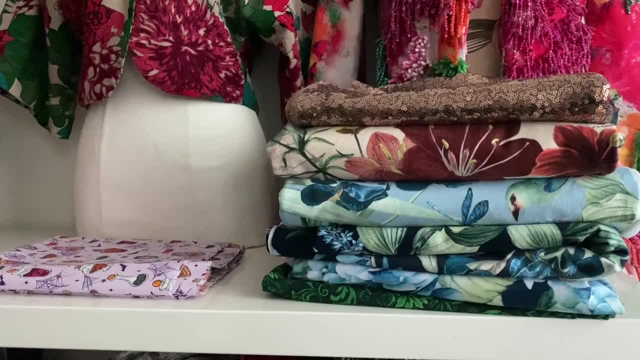 So now I can do both because, yes, I was just running so short of jackets I really needed to buy another bit of fabric. It's ridiculous. Now I've rearranged the side bench, So the jackets in front of the Kandinsky jacket are the ones going to use that pattern. 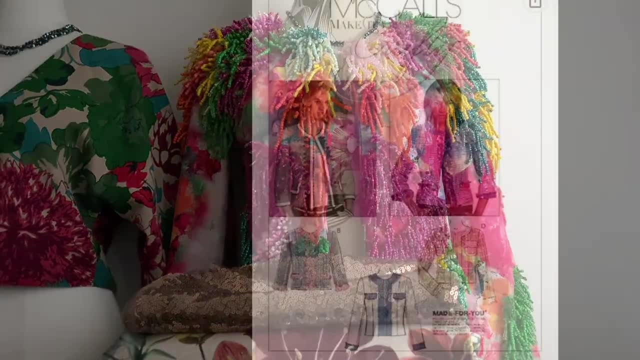 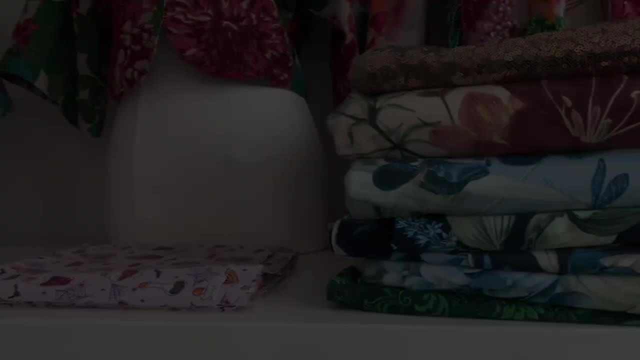 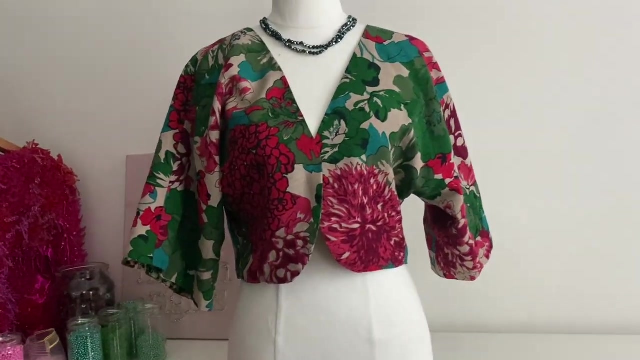 the discontinued McCall's Chanel style jacket, and the jackets and the fabrics in front of the middle jacket are the ones I'm going to turn into a reversible cotton summer jacket. I put the lemon vintage print there just to bulk up the pile. Yeah. 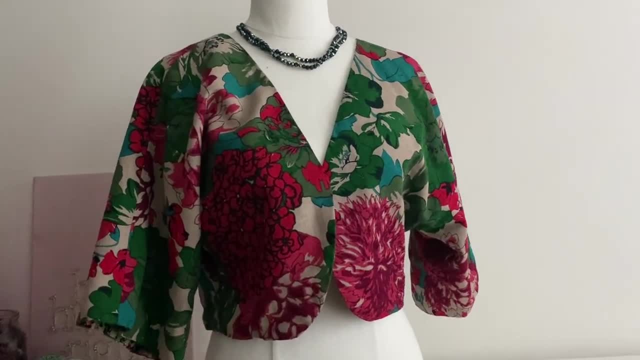 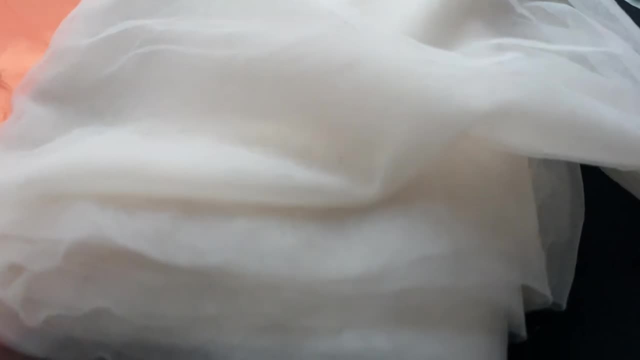 Two bits of fabric, that there are loads of other ones, but they're aside. So then I I think I've told you about my absolute love of beige tulle. It's just that when I was a, when I was young, I worked in a 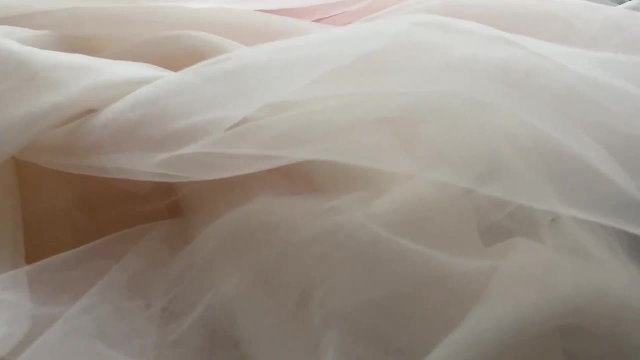 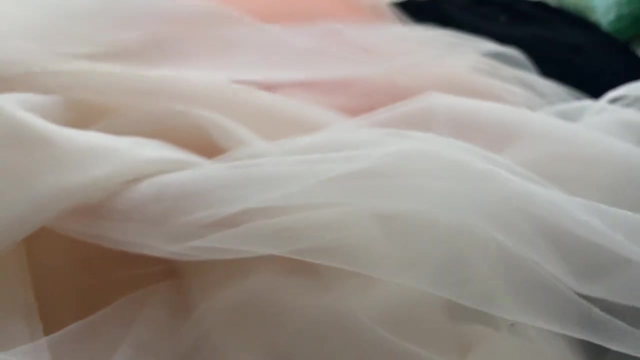 uh, like a really good florist store that did the expensive weddings, And so you got to see pictures and fabric samples of loads of wedding dresses like so many, and the vast majority of them are either white or cream, and it gets a little boring after a while. 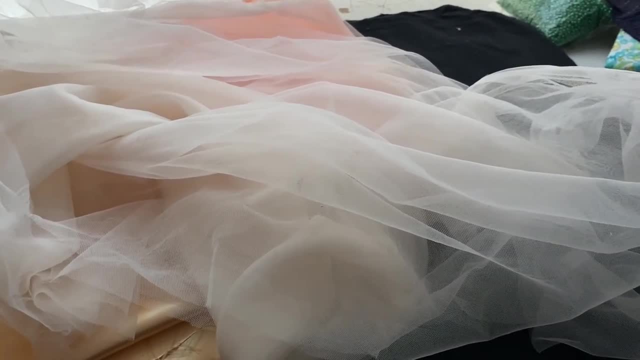 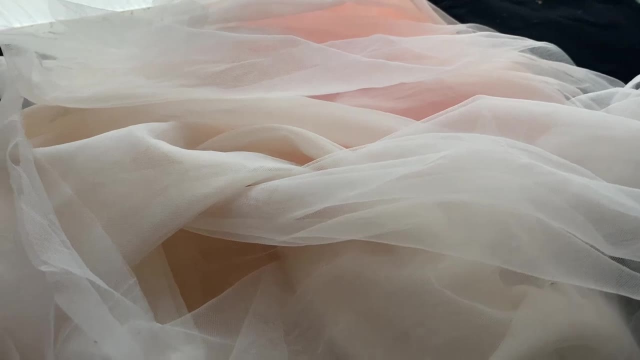 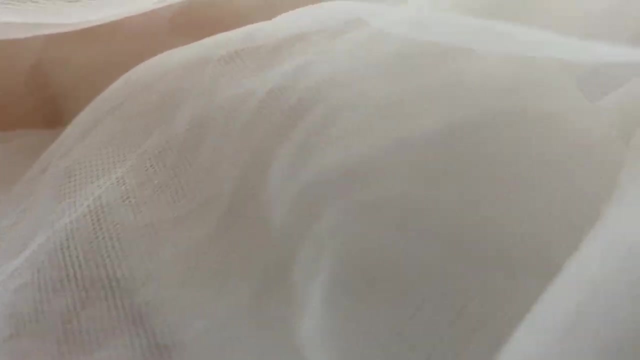 but every now and again you get one of the beige Vera Wang ones and, oh my gosh, they are just the most beautiful wedding dresses in the world. Like Vera Wang is obviously she does proper like collections, but she also she's really popular as a bridal designer. 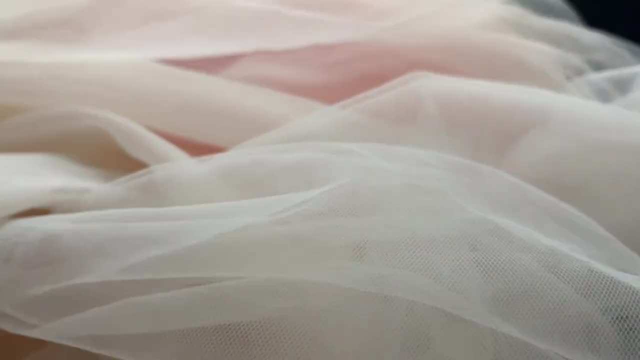 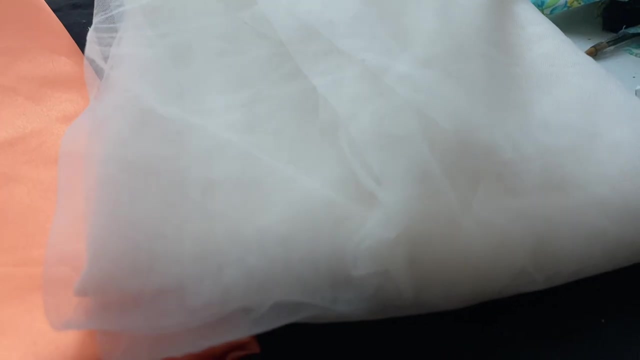 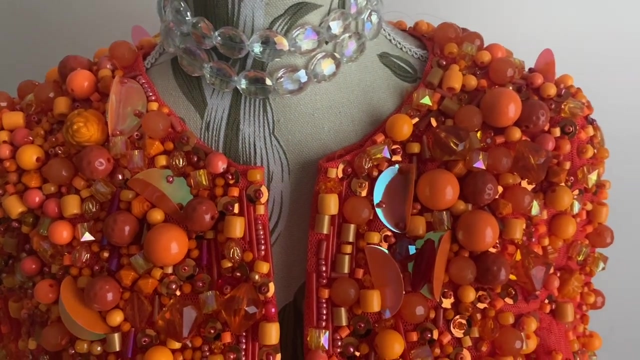 So she does these a wedding, a couple of wedding collections, each year as well, And those dresses are just amazing. So anyway, um, yeah, that I bought the beige for um, I'm actually going to use it to do lining for the orange beaded jackets. 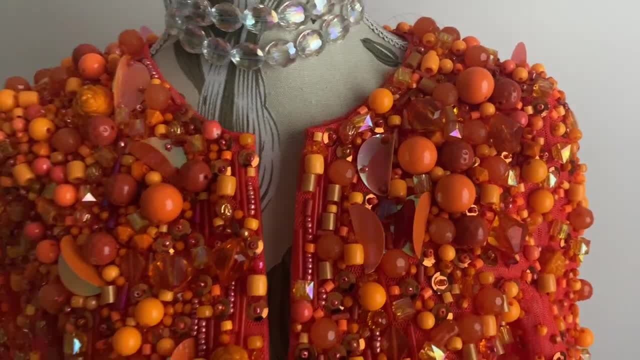 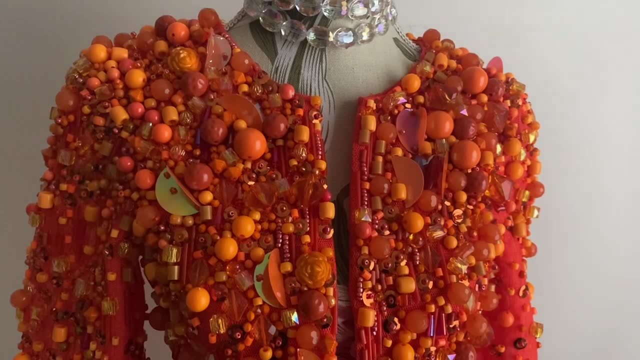 Oh my gosh, I have to set aside a week at some point to just make silk lining for all the jackets that I finished the outer jacket for, but I haven't yet done the lining for silk. Like you need to get your silk pins out. 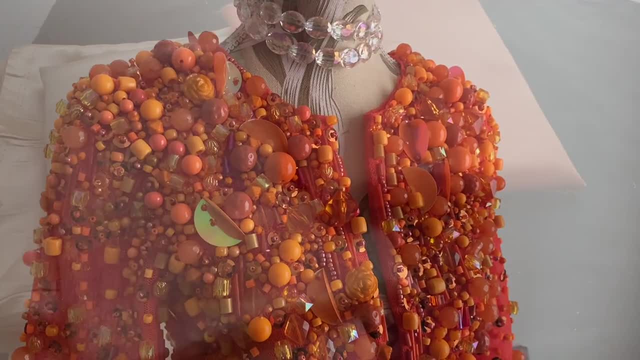 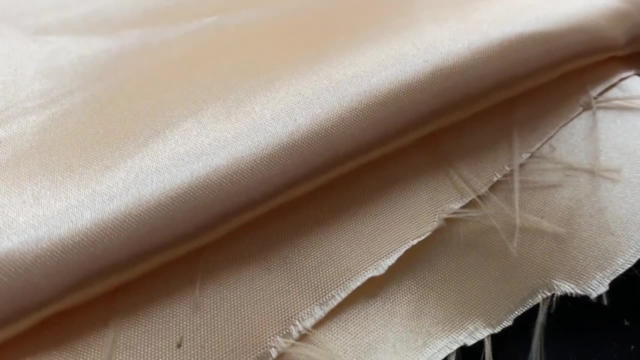 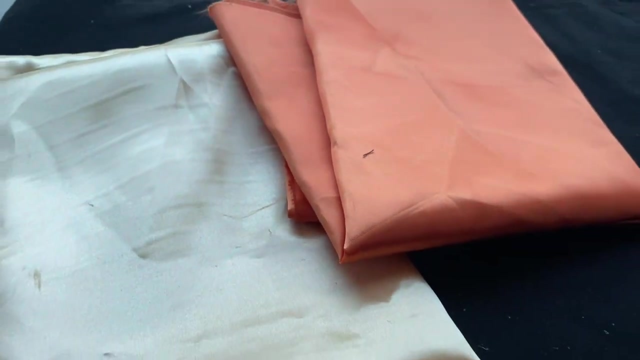 You need to get your silk scissors- special scissors for cutting silk. You need to put us microtex needle in the sewing machine. It's a whole thing anyway. So, um, I've got two fabrics left. Originally I got. there's a whole backstory to these two fabrics. 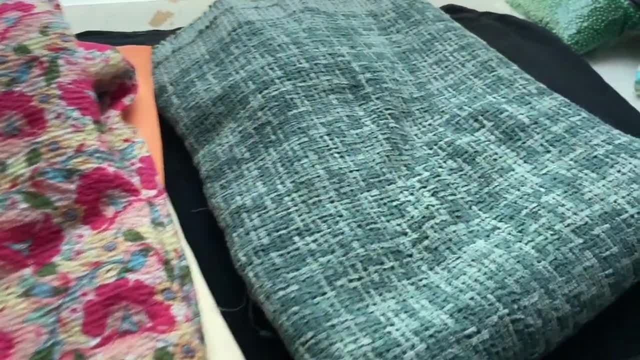 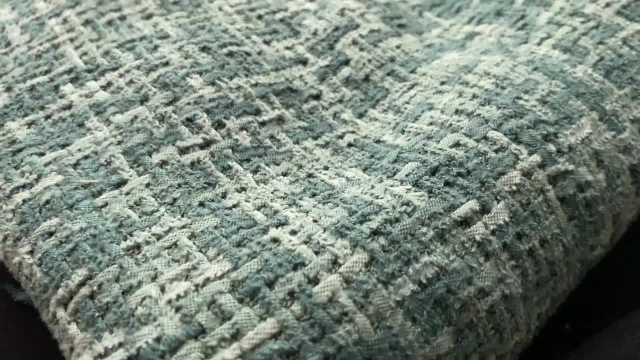 They're sort of synthetic. They're not silk, They're satin synthetic, whatever it's called. So anyway, for pretty in pink. I was going to make pretty in pink The main character, Andy. she wears a lot of pink. 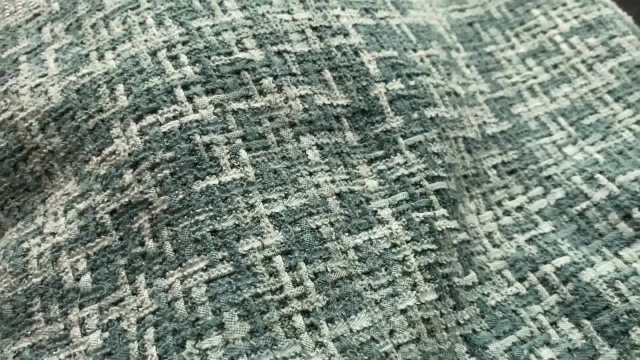 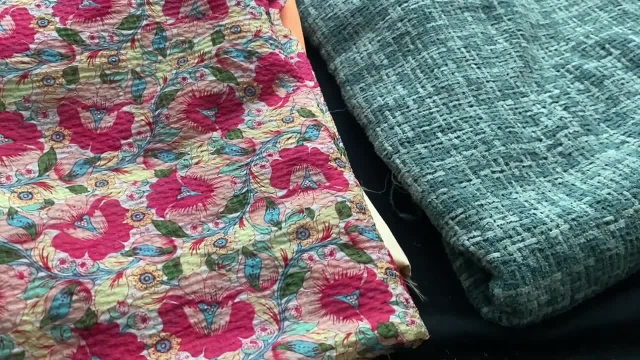 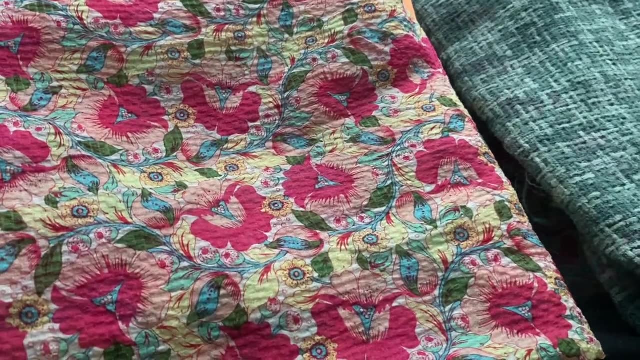 but also some teal and aqua, So I was going to make this tweed jacket. I bought this fabric in New York years and years ago And more recently I bought this absolutely adorable silk to go with as the lining, because I just think they look perfect and it'll go perfectly with the pretty in pink capsule collection. 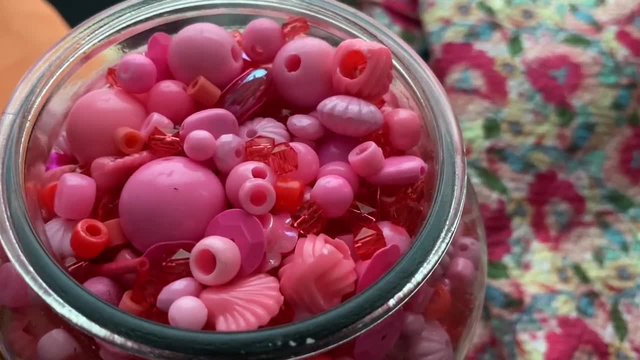 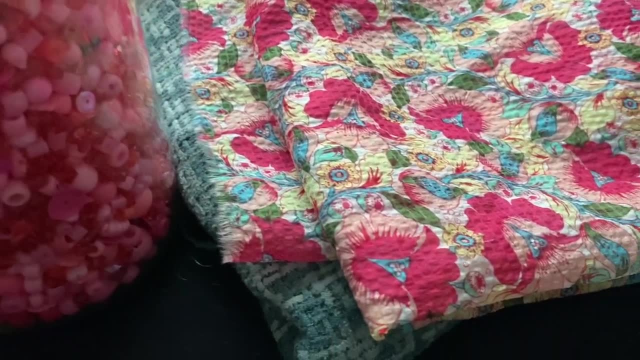 But then so I had that silk lying around for that And I happened to get these beads out there in a bag and I had to get something that was under them, And these two ended up beside each other And I was like, Ooh. 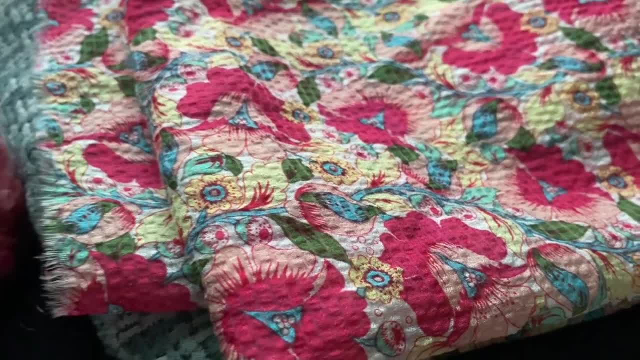 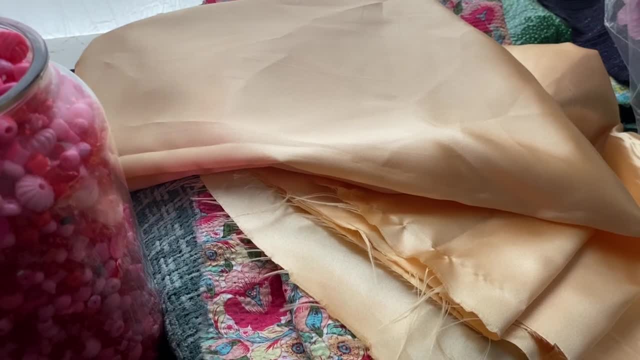 you know those. there's a rose called a peace rose and it's a yellow rose and it's got hot pink along the edges and it sort of fades to a pale pink. Then the rest of the rose is golden. It's just the most beautiful rose. 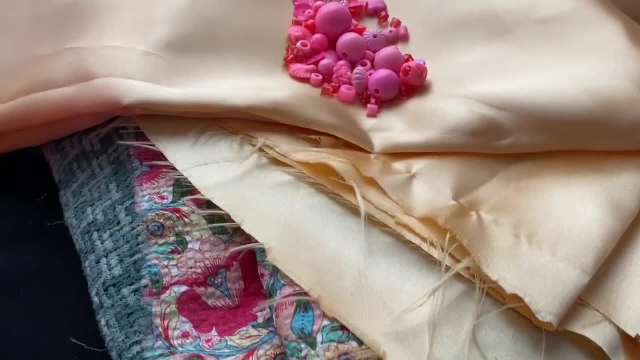 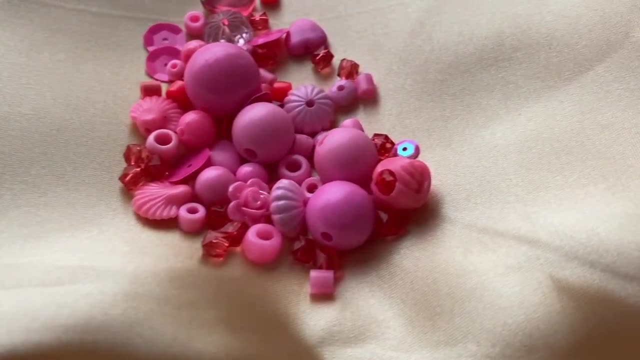 but also it's called peace. So I bought just a yard of this satin looking fabric and I was going to make the base jacket out of that and then overbead it with all these bright and hot pink beads, And conceptually I love the idea. 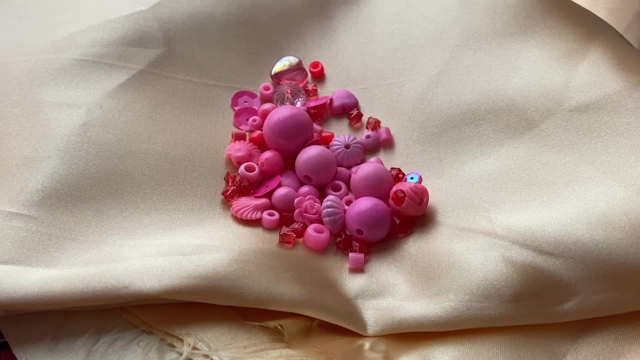 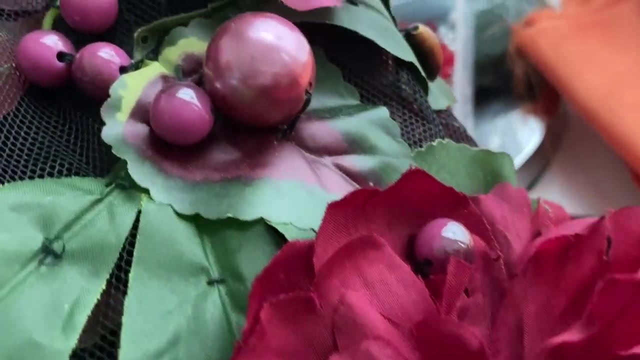 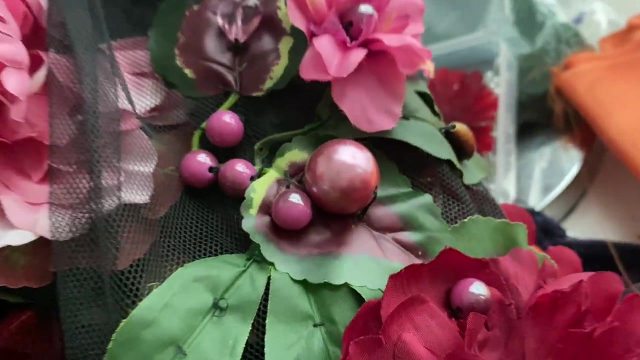 I absolutely love it, but I just don't think it's going to work. like, what color thread are you going to use? As you can see here, like I've used black and dark green? Um, well, I've used black and a wine colored thread on most of them, and then green. 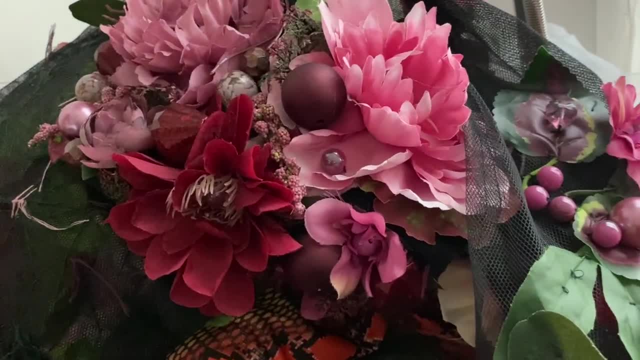 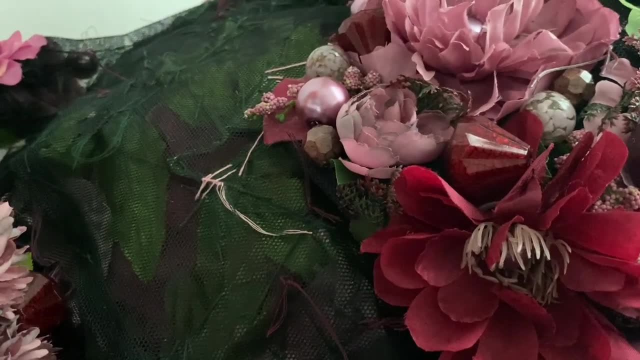 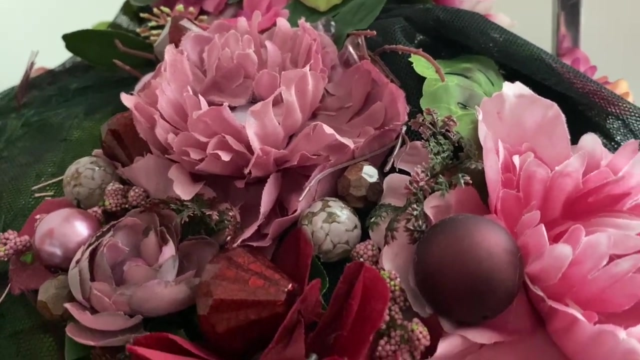 black and green on the darker green and then two different greens on the green and mauve sort of- um yeah, a dusty mauve colored thread on the. So my point is that you have to use a thread that blends into the base jacket and works well with beads. with this. 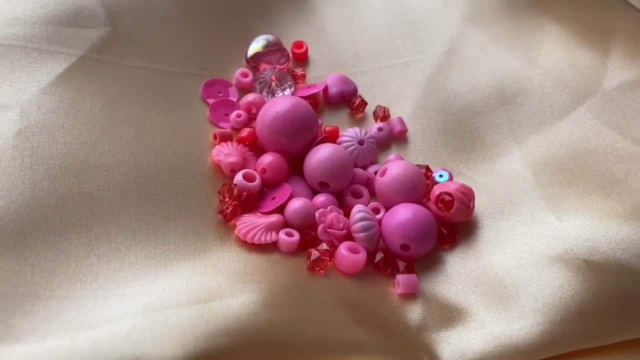 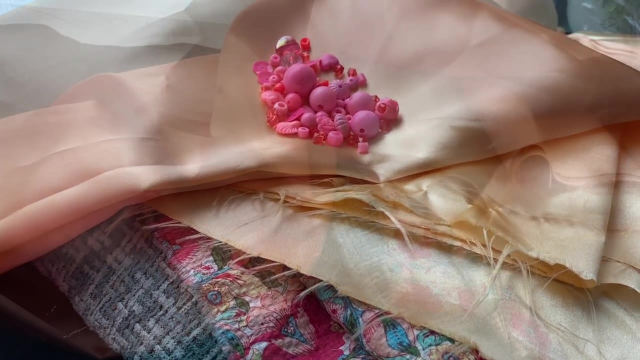 What do you do Like? either it's going to blend with beads or it's going to blend with the jacket, and either way you're going to be able to see the thread and it's just going to be a little bit jarring. It's not going to look like, in my opinion. 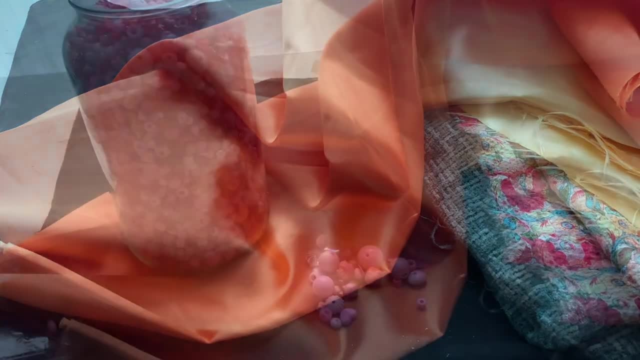 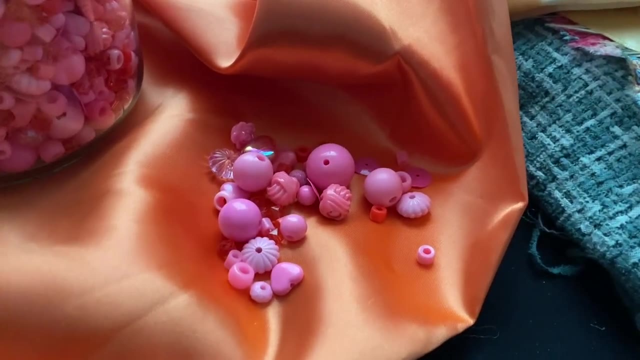 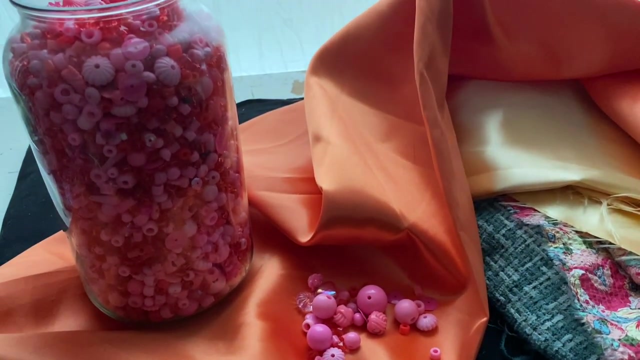 a jacket with that's beaded or embellished Um and yellow was should look effortless. You shouldn't be able to see how much work went into it, Whereas when you could see the thread it just sort of makes you reminds you that there was a human being who worked on these four tens or hundreds of hours. 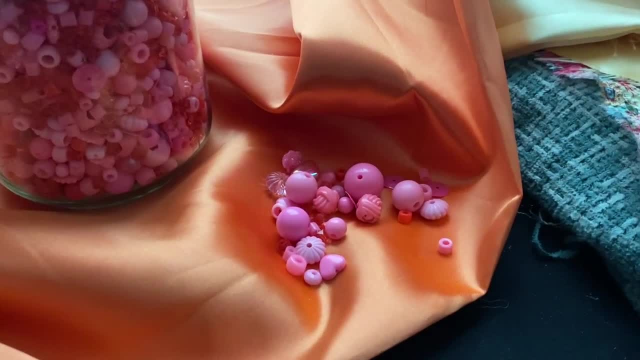 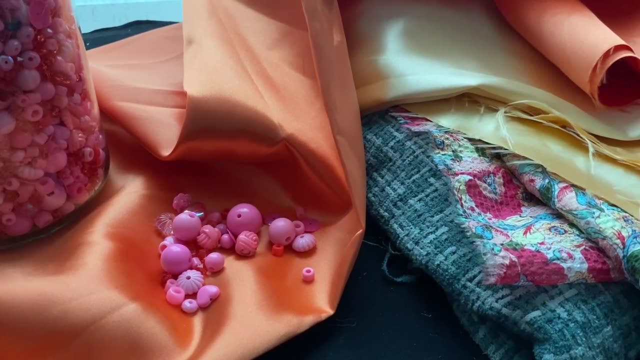 And sort of that's how it was created And I like it, I prefer it. you know, um, when you go to the ballet and you know, the dance to just sort of flies up into the air and the guy catches a sort of thing and it just looks completely effortless. 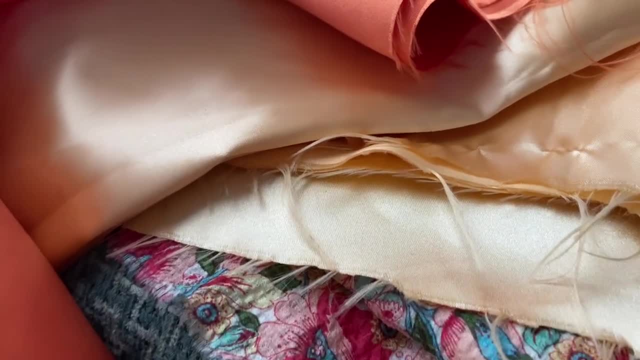 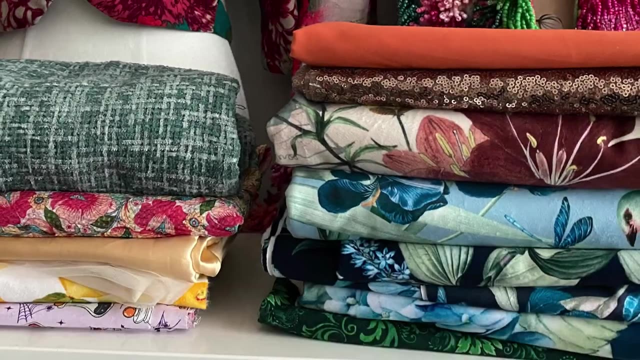 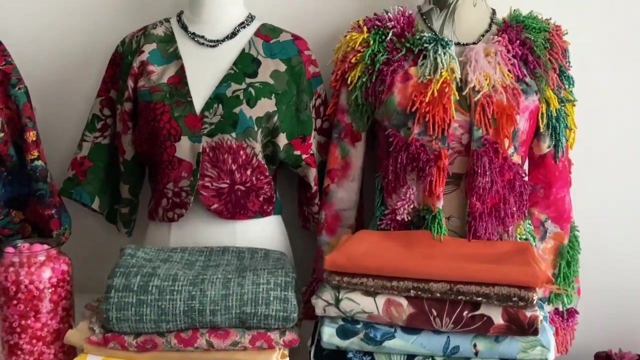 what I love. so I was. then I got the orange and um, yeah, I think I'm going to make the jacket out of the orange and have the hot pink on that. and I've got loads of golden beads so I can do golden beads on the gold. but yeah, that's the story of those two bits of fabric. so there we go. that is my um. 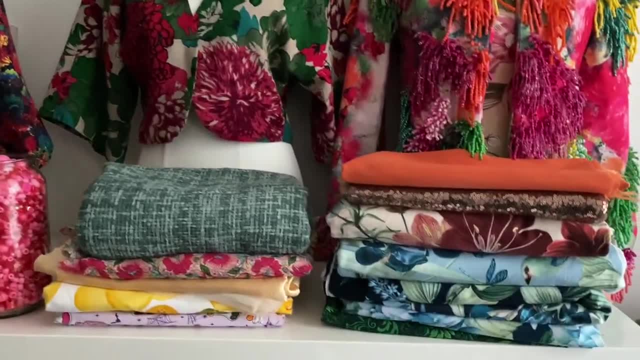 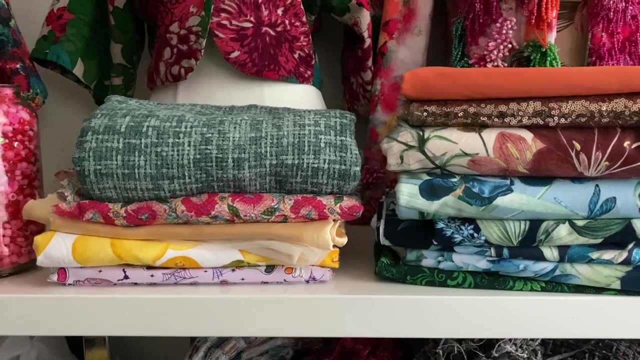 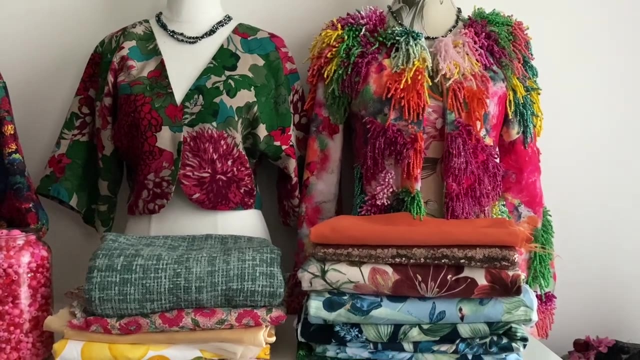 fabric haul and, yeah, pretty much just jackets and a dress. someone's um- someone was new to sewing uh YouTube, and she was sort of just making a list of other other um channels that she's watched and she's talked about mine. she's like, yeah, she only ever does makes like three things. 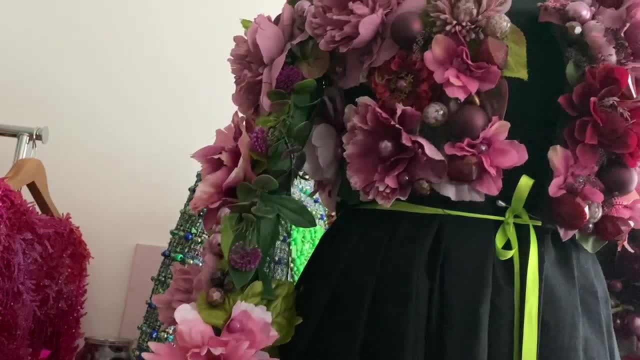 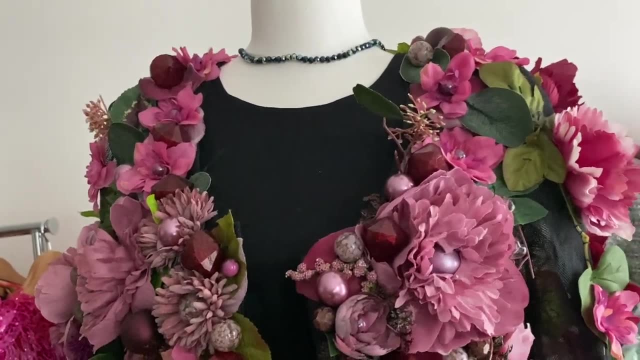 but she makes them in the most widest variety of ways. and I was like, yeah, I kind of do, don't I? but like, if you know what you like, then I mean, I did when I was younger. I just worked through loads of different patterns and then I just donated them after. I was like, not, don't like. 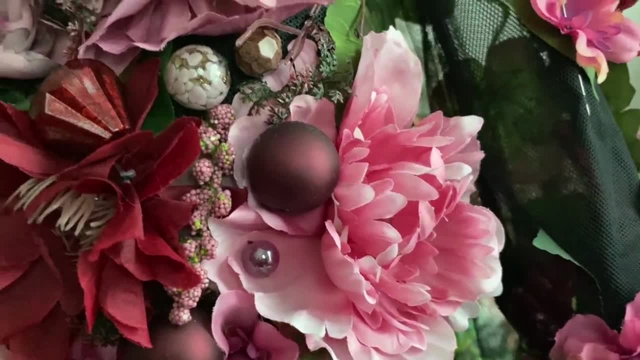 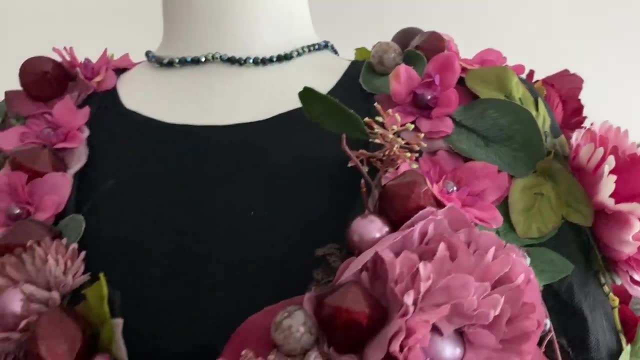 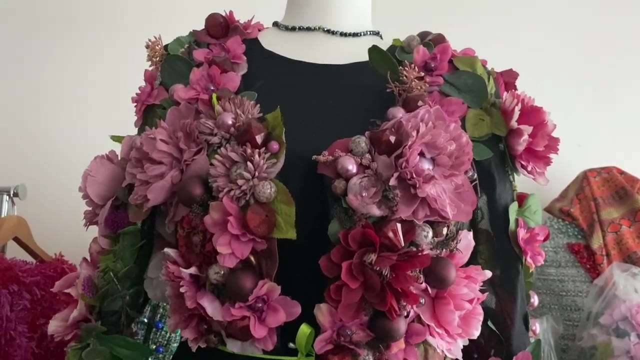 that pattern. and now I'm sort of, yeah, you sort of find the ones that you really like, the patterns you like, and you just sort of do endless variations on the ones you like, and, um, so this is a jacket that is still unfinished, and so I got out all my flowers and so we've turned. 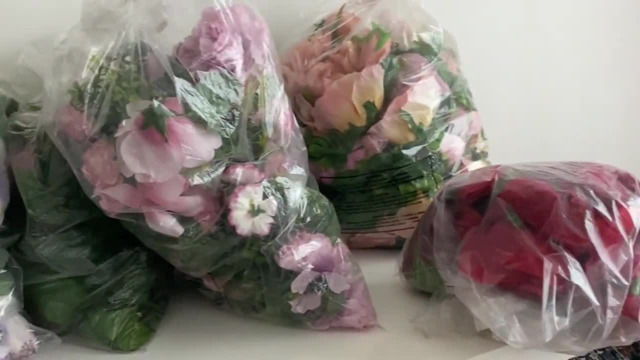 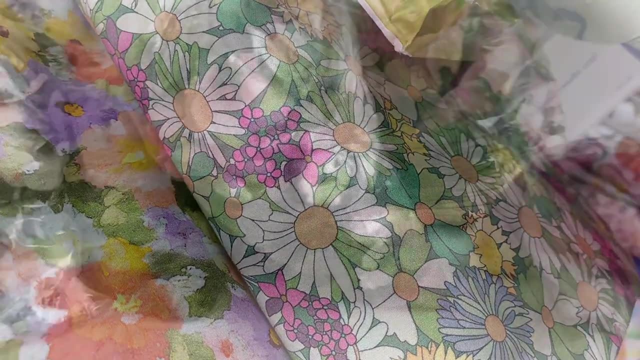 into a bit of a sewing vlog now. no more new fabrics to show you. well, there are some, but I'll. I'll show you another visit to a fabric store before I show you those fabrics anyway. so, um, my wine colored floral jacket. I need a few more. 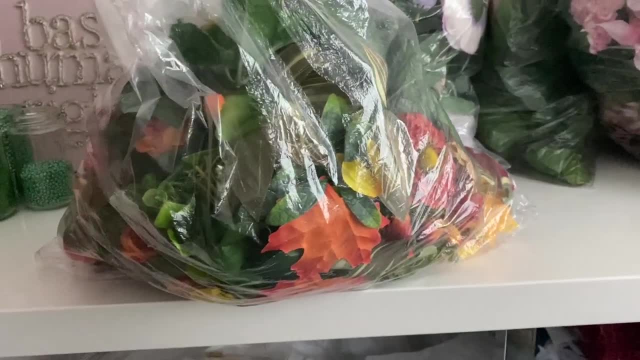 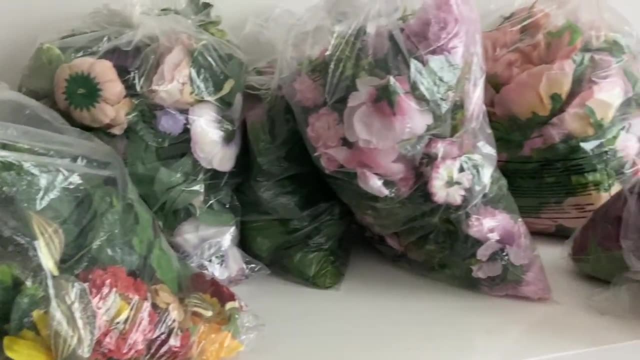 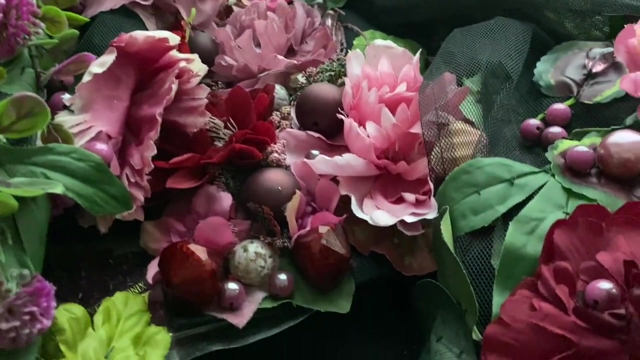 flowers to finish it. um, because I've got, like I think I've got four or five more flowers, but I actually need like a dozen more. so here is the jacket. I've laid it down on my workbench so we can match the colors, and I've got out a bunch of other bags of flowers that I've put. 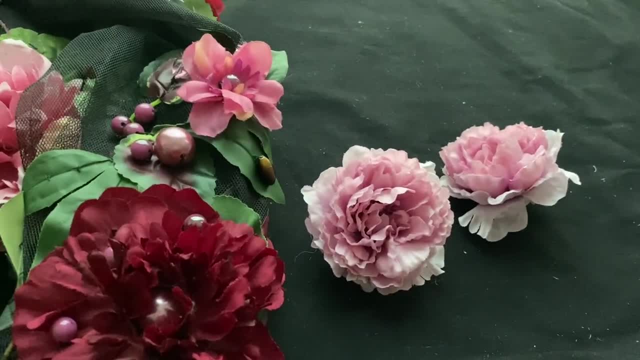 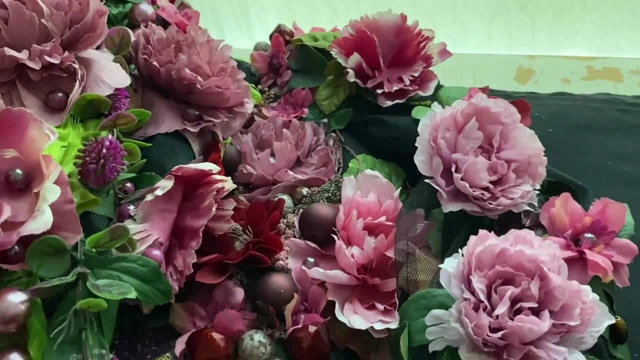 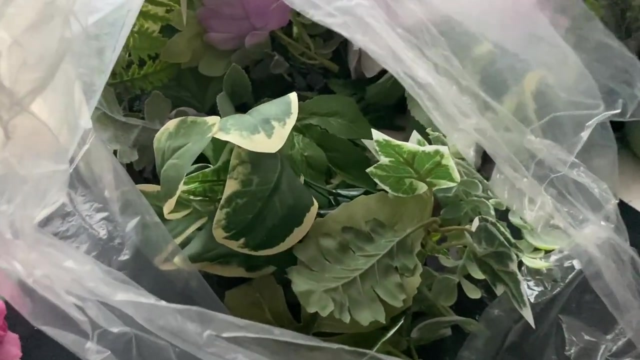 aside to make individual jackets out of, but I'm just going to steal a few flowers from each of those bags and hopefully I'll be able to cobble together enough flowers to finish this one. so, um, this one is more gray mauve and um pale green like sage colored. 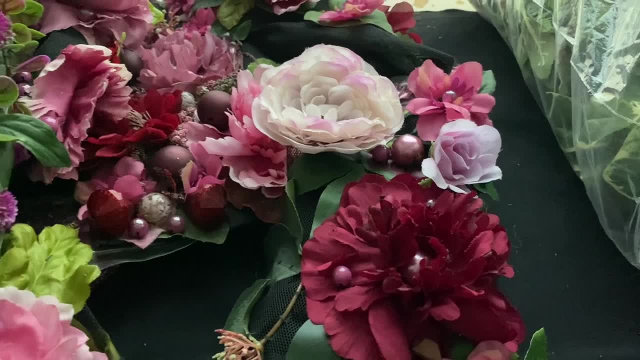 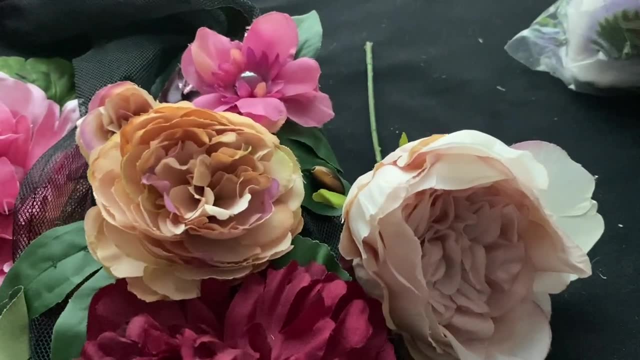 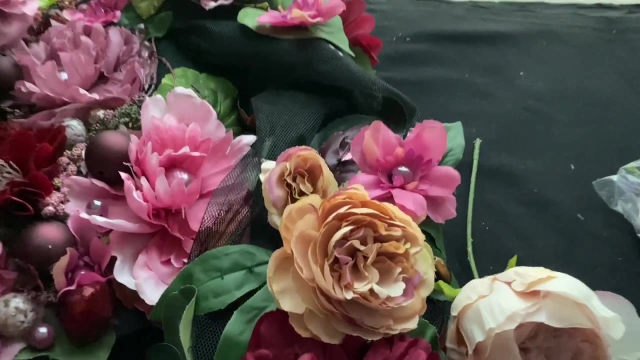 greenery and yeah, no, I don't think they go at all. however, these ones here, um, I don't like the one on the right, but I do like the sort of brownie colored one. I think they look quite good. maybe, I mean, they definitely look better than the mauve colored one. 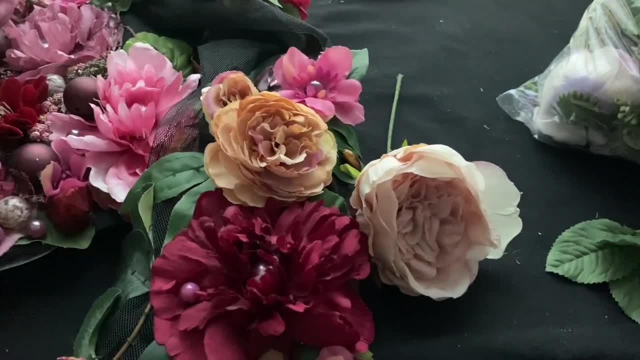 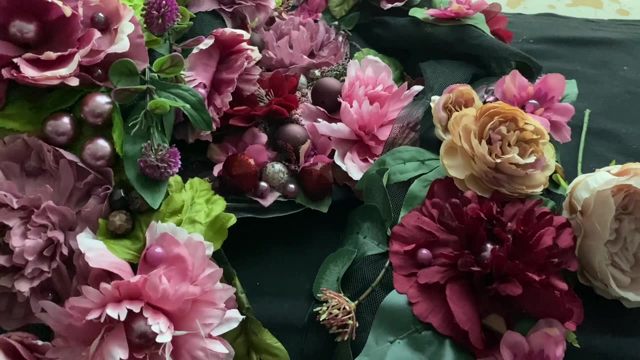 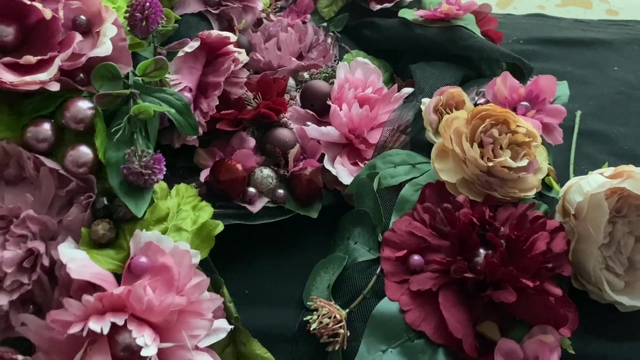 anyway, they're interesting. see the jacket that I'm working on. this wine color jacket has some twigs and branches in it, so that's why I think the brownie colored roses might look good. it's usually called antique color roses, but I don't know. this is me like I nestled it in between. 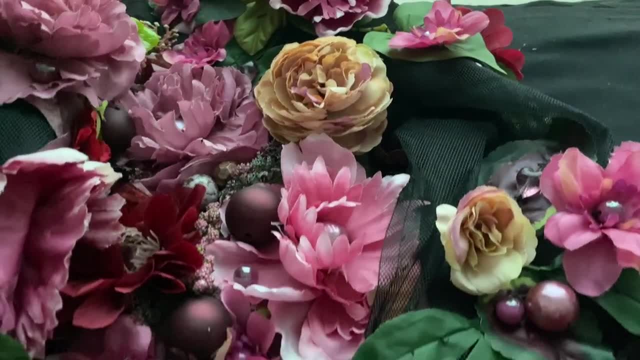 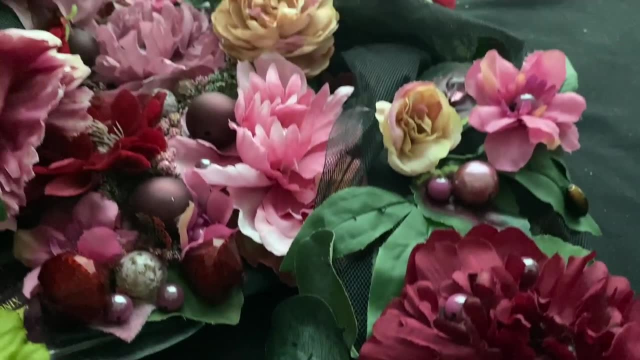 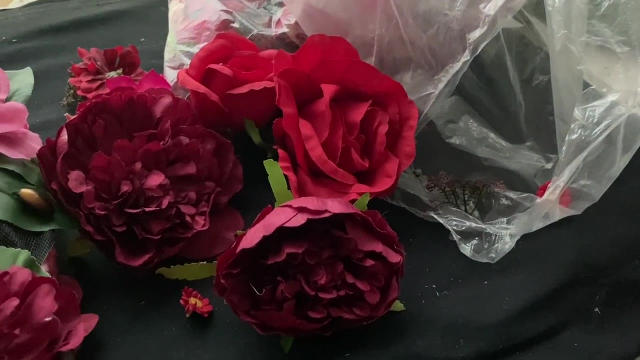 the other. see there the seed pods, and there's also some branches a little bit higher up, brown branches. I mean they're definitely interesting, so I kept them out for a bit. then the next bag was red and wine red, like a darker red, the brighter red. uh, yeah, I don't think they go well. 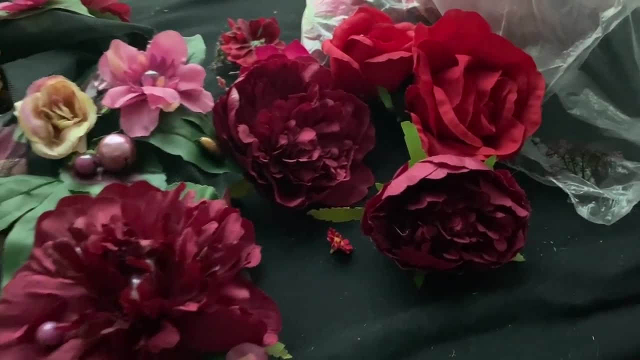 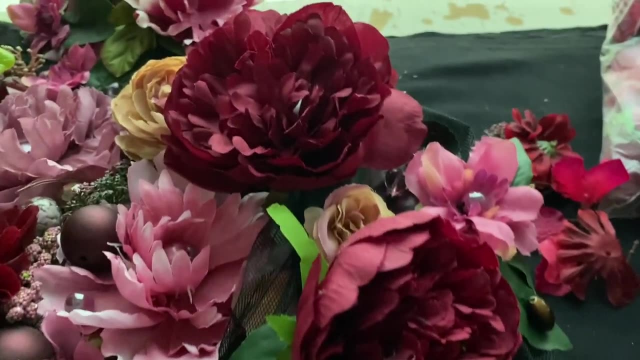 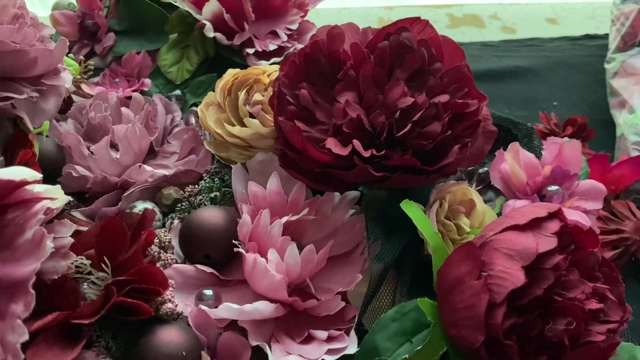 with the lighter colored. yeah, they don't go well with the dusty mauve colored ones or the the the brown colored ones. so I have to make a choice. I think I would prefer the wine, the dark red colored ones, and the dusty- um whatever wine colored ones, and maybe I'll take out the brown ones for now. 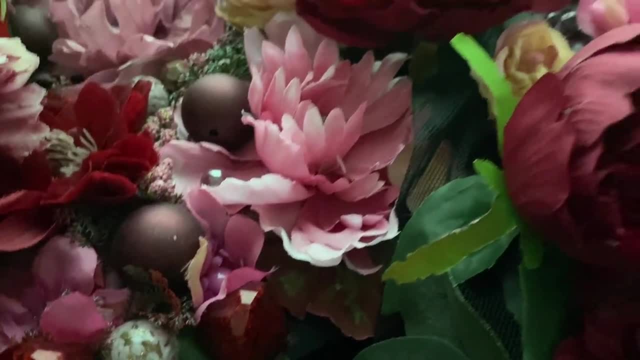 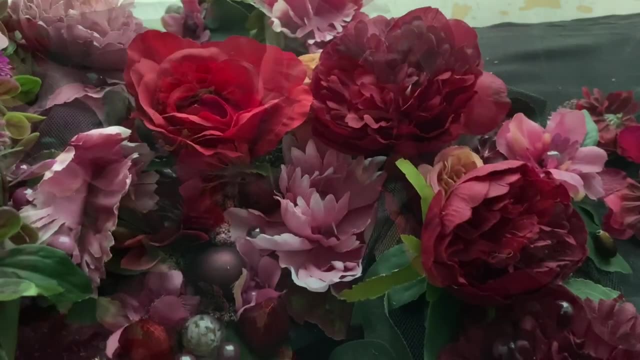 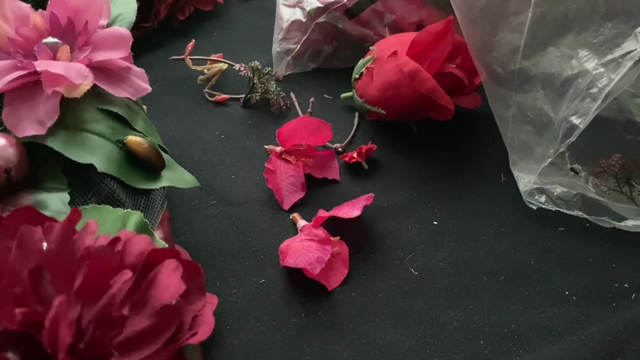 and yeah, I do think the the dark red ones, the really deep burgundy ones work well with the bigger beads that I have and those big beads. sometimes I buy the most ridiculous beads and like they're just such a challenge to use. so, yeah, I really do need to get something that ties them. 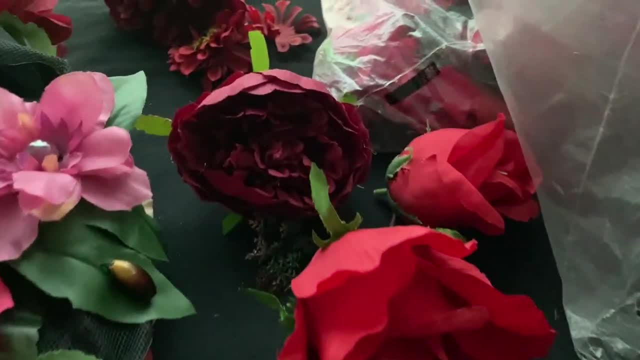 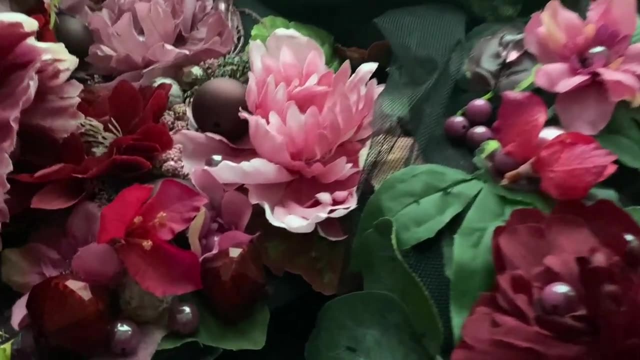 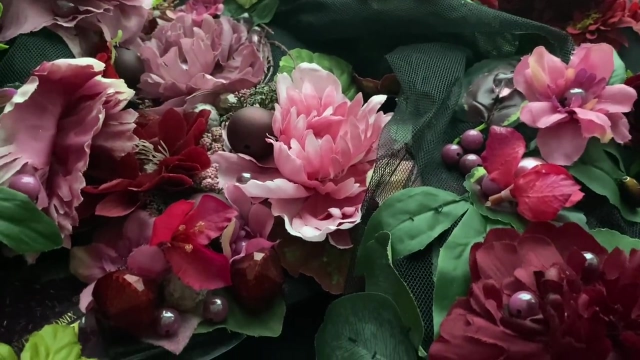 better more into the jacket, because the beads are a bit too big and a bit too noticeable at the moment. so I also have some little brackets, um little bougainvillea flowers. they're not. I know they're not flowers, they're brackets, um, but um. yeah, we'll just call them flowers and um. 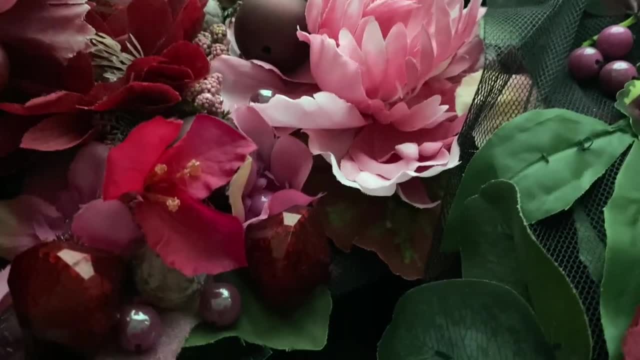 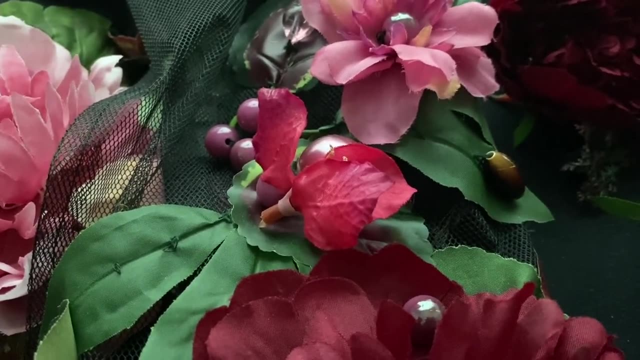 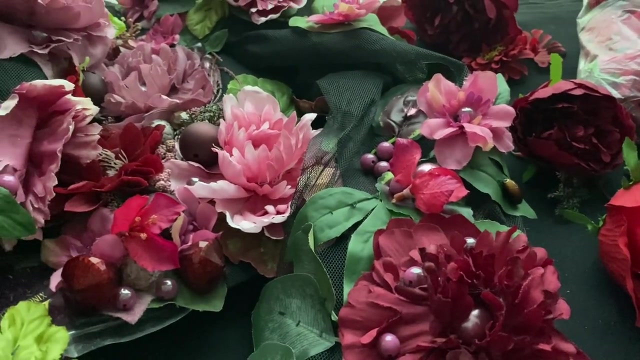 I think they go well. I mean, it doesn't exactly go like it's more. it's sort of a dusty magenta color and it doesn't really match anything but it all. but it just sort of it makes the dusty, um mauve colored ones seem like a softer, more glowing color. 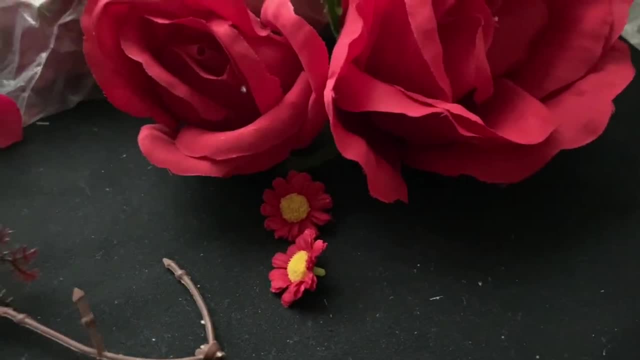 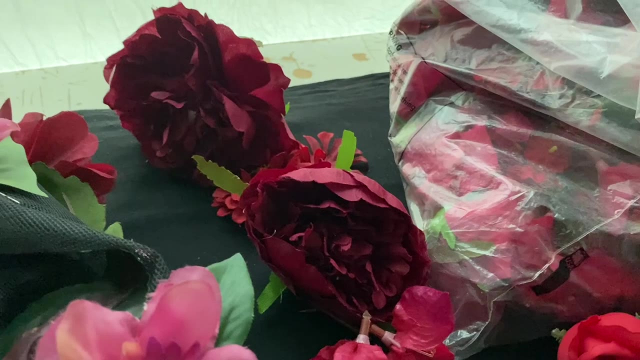 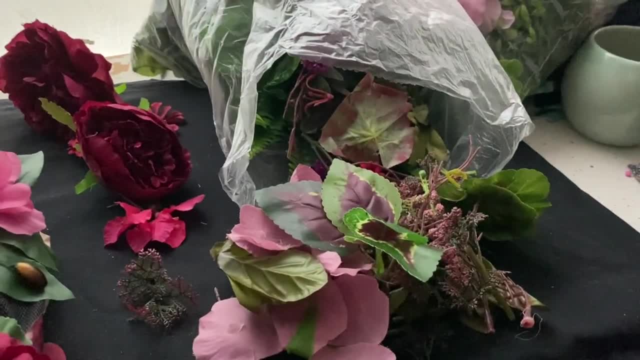 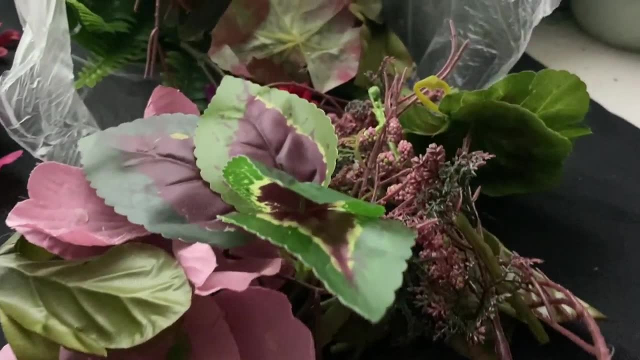 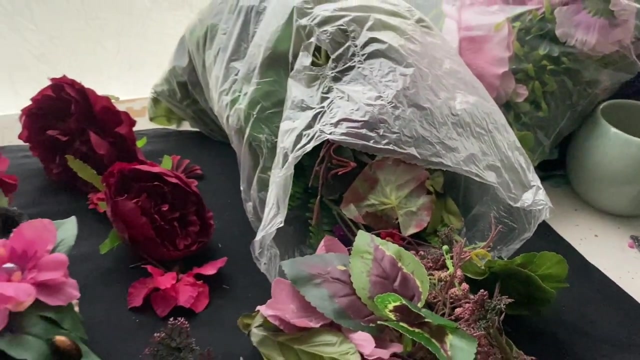 so we're going to keep those out. I think they're going to work well. and then this is just the leftover bag of like. there's a couple more um dusty mauve roses and lots of two-tone um leaves that I still have to stitch onto this one. so this is the bad. this is all that I've got left. 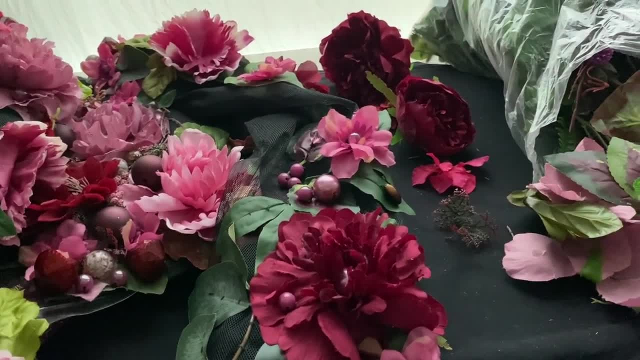 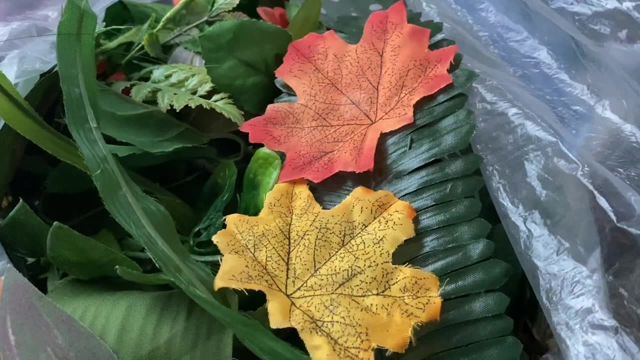 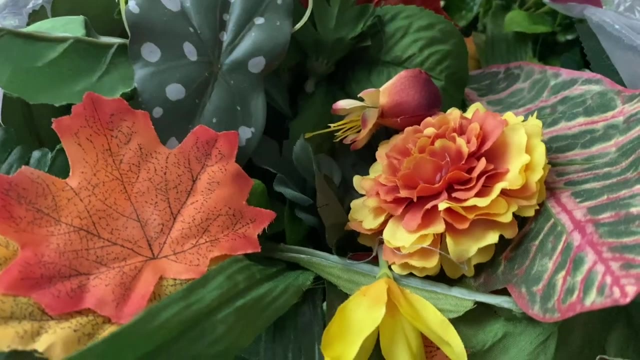 though. so, yeah, I really did need a couple more flowers, so I ended up- and I do have this bag of autumn harvest, one with the um. those are the autumn leaves that I have. they're absolutely gorgeous. I've got like 50 of them, so that's going to be quite the jacket, but yeah, and I've got some. 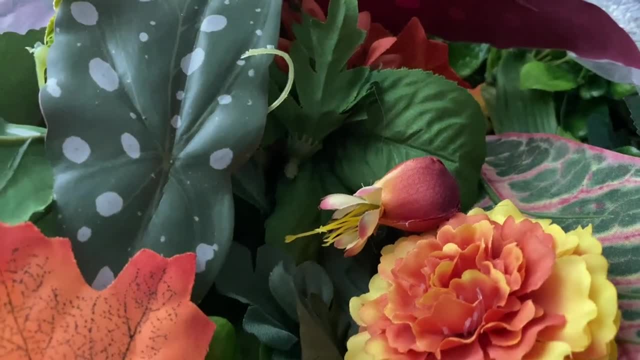 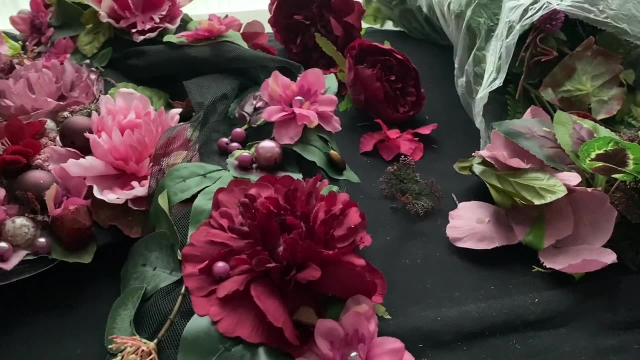 rose hips and some seed pods and things in this bag, but I think I'm going to leave them in some little branches and twigs and things. but I think I'm going to leave them in that one. and in October I'm going to do an autumn harvest one. I'm really actually looking forward to making that one. so 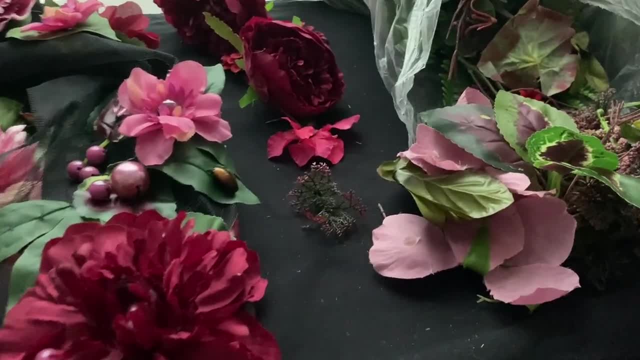 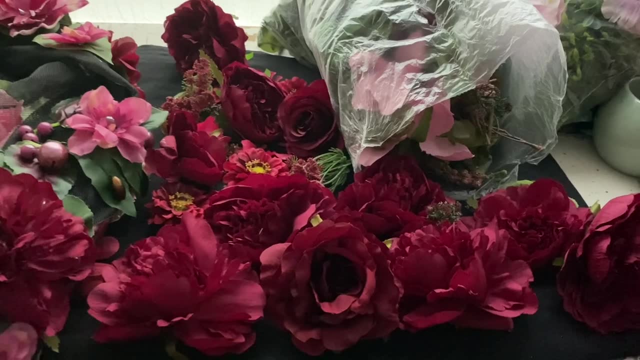 I'll leave that one as is and I'll see you in the next one. And yeah, I think I've got enough now that I sort of went through that whole, um, dark red bag and got out a dozen or so of those ones, just gave up on the idea of making a. 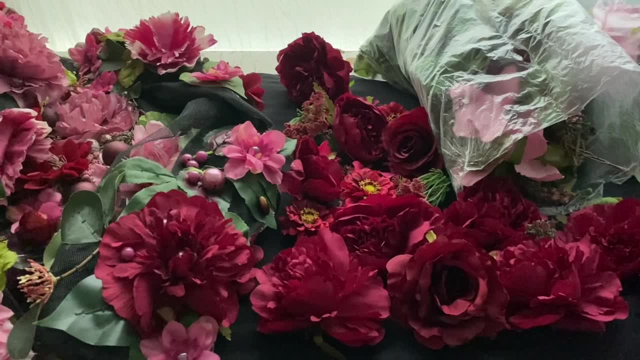 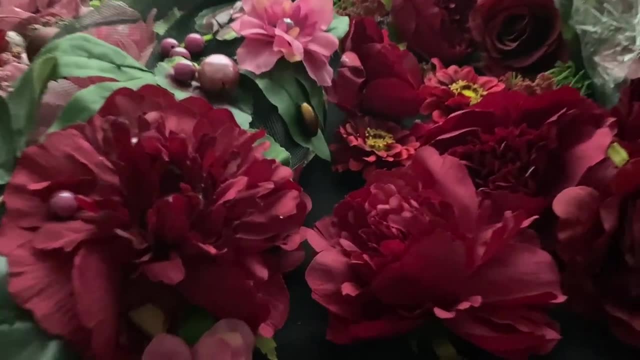 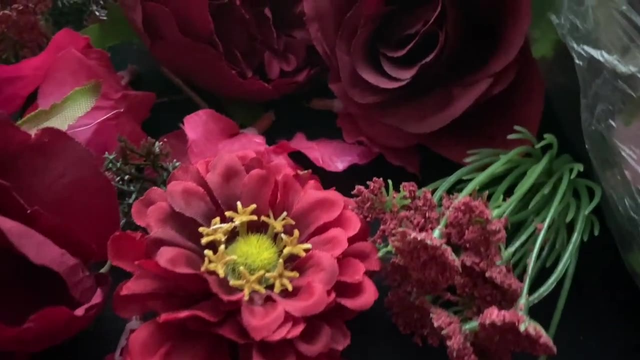 um, because I did start the red and dark red jacket and it just doesn't photograph well, whereas if you put the dark red flowers with the dusty, um, burgundy ones, they actually the camera can discern the difference between all of them, whereas if it's just red and red, 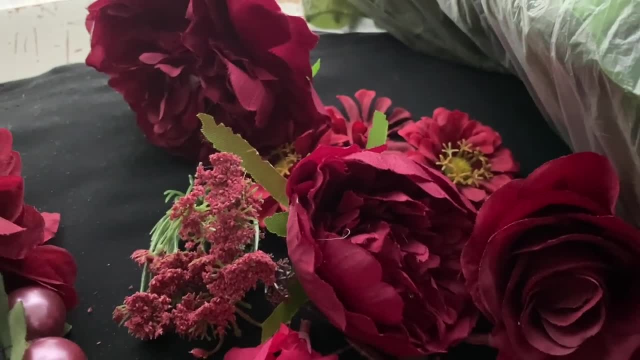 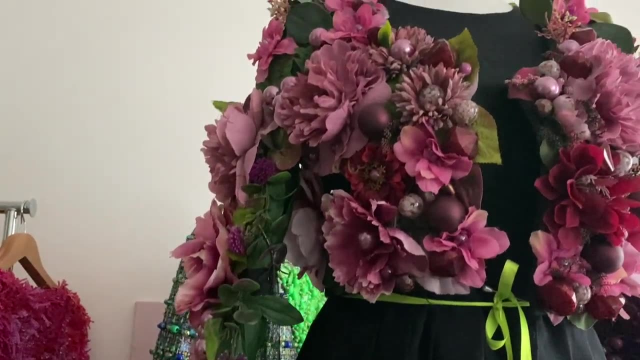 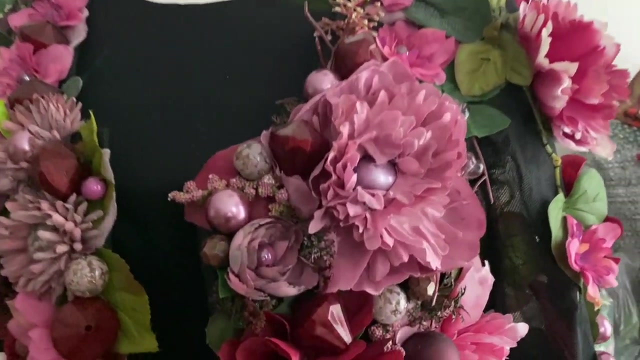 then the camera. yeah, cameras just do not like red. in well, I can't get my camera to like red, it has to be mixed with other things. so, yeah, I think I've got enough flowers to finally finish that jacket. damn, now I can't procrastinate anymore. but um, yeah, so there you go, that is. 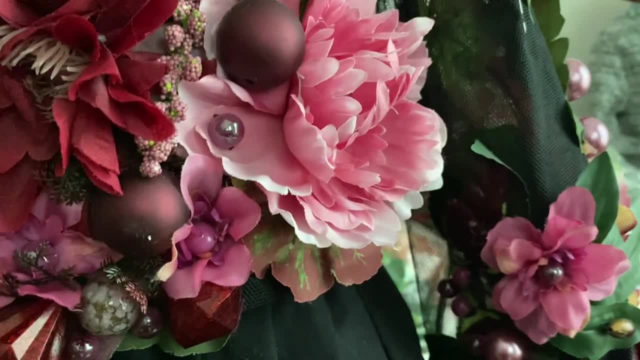 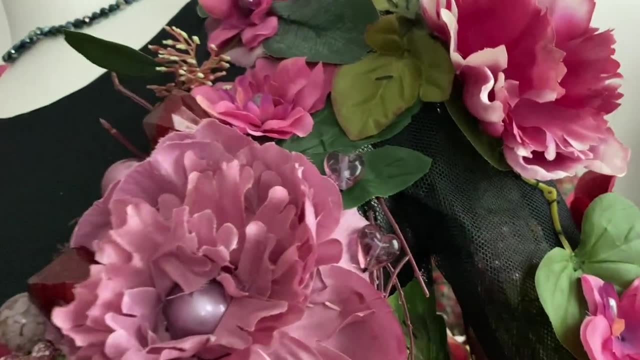 the end of the episode. I've got some lovely fabrics to make jackets and one dress from, and I've got my flowers sorted so I can finally finish that flowering. Anyway, thank you for watching. I hope you've enjoyed. I hope you've been inspired to rummage. 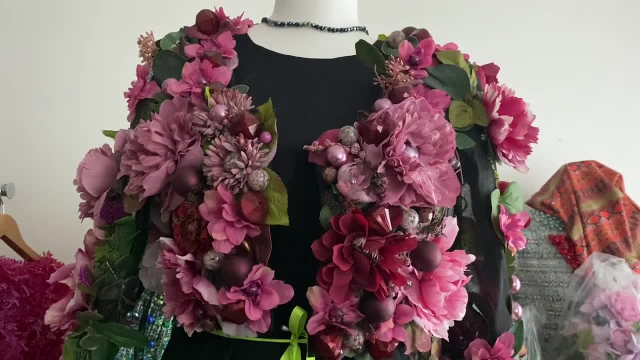 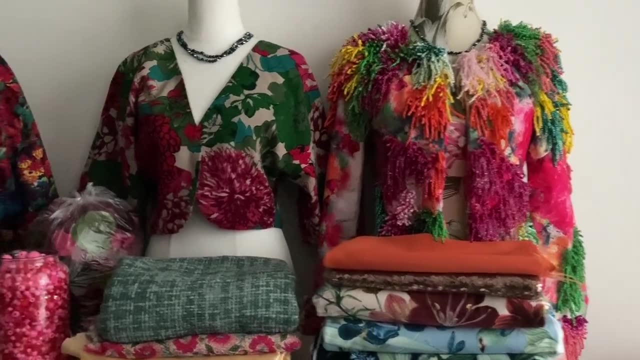 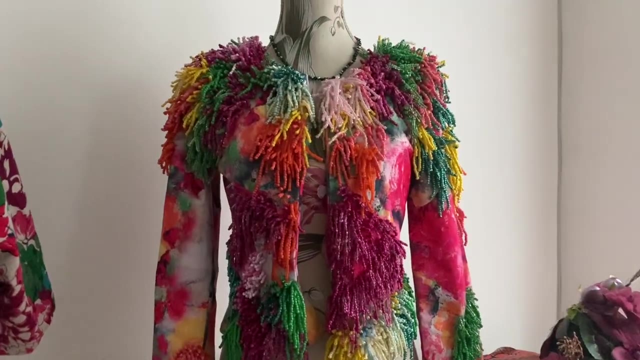 through your fabric stash and make something out of one of your challenging fabrics. I haven't had the Kandinsky out in a while. I still am just so impressed with the way that one turned out. I bought that Kandinsky- that um sort of decorator velvet fabric, on an absolute whim, like I had.